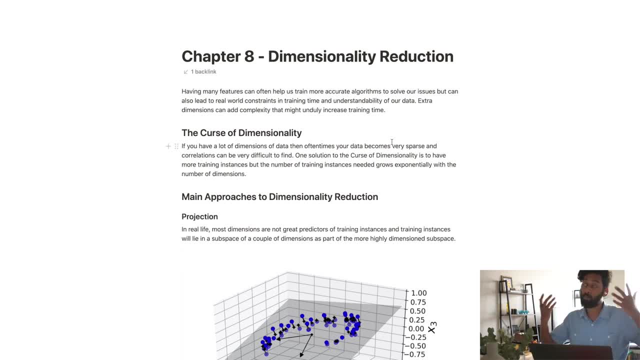 keeping up with what we've been doing so far. you'll know that oftentimes in well in machine development. we'll have a table and in that table we'll have multiple columns And each of those columns represents a feature or a dimension. So, for example, if you have a dataset with four columns, 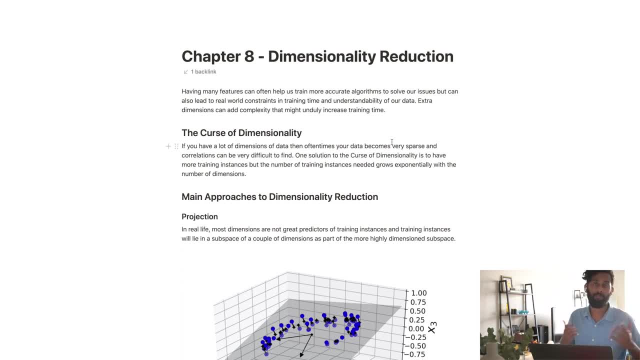 where one of them is the column you're trying to predict. that's a three-dimensional dataset. It has three features and then one column you're trying to predict. So, when we go through dimensionality reduction, what we are trying to do is we're trying to compress the number of features. 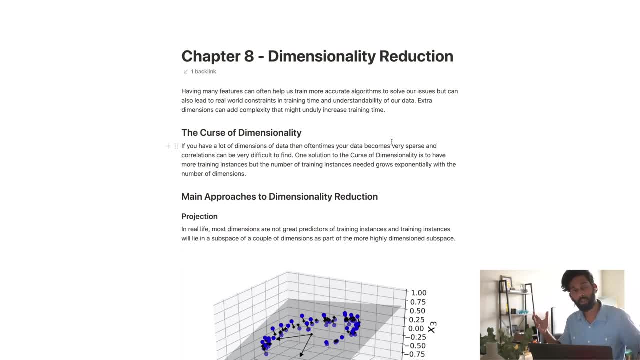 from you know, maybe 30 to 100 to 500, down to maybe a couple of dozen or even a couple of hundred. if you have enough features In sufficiently complicated machine learning applications, you'll see that people tend to have hundreds of columns And you can imagine why we may not want to actually. 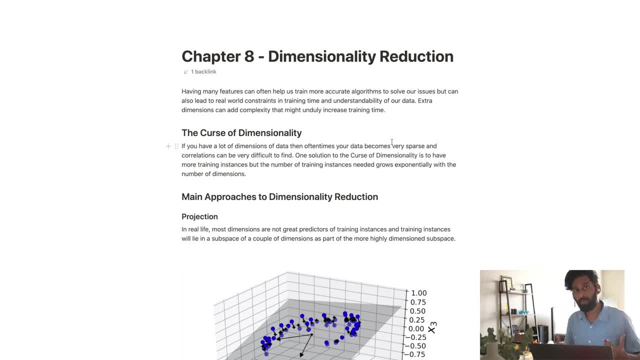 model on all of those columns. Two main reasons that you want to use dimensionality reduction: One is because you might want to visualize your data- And you can't really visualize data outside of four dimensions, And I'll show you what I mean in a second. And two because you might have 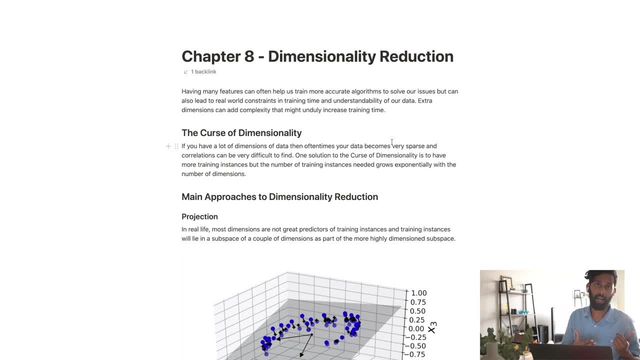 difficulty putting a large amount of data into a machine learning algorithm without intensive computational resources, And the benefit you might get from the last 100 columns may not be worth modeling on the extra 100 columns. So those are the two main reasons you'll want to reduce your. 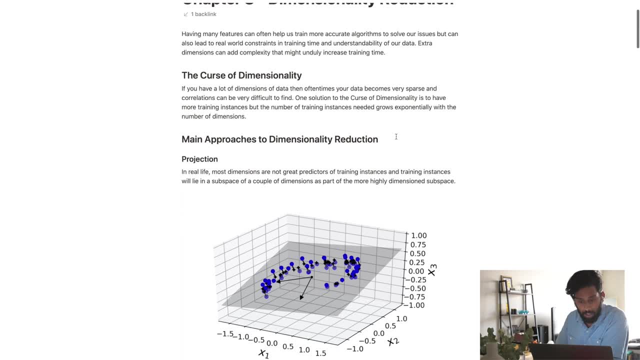 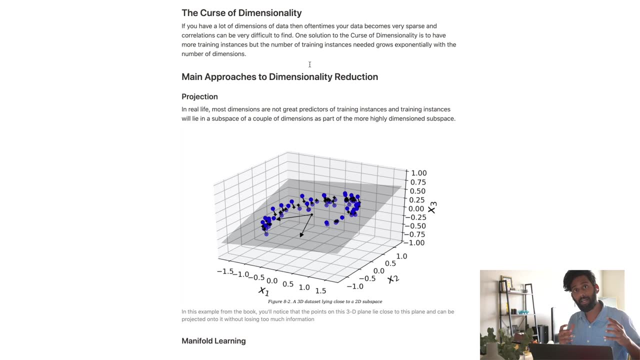 dimensions. So let's get started with the chapter. So first they go over something called the curse of dimensionality, And if you have a lot of dimensions of your data, then oftentimes your data becomes very sparse. And what they say is that in real life, 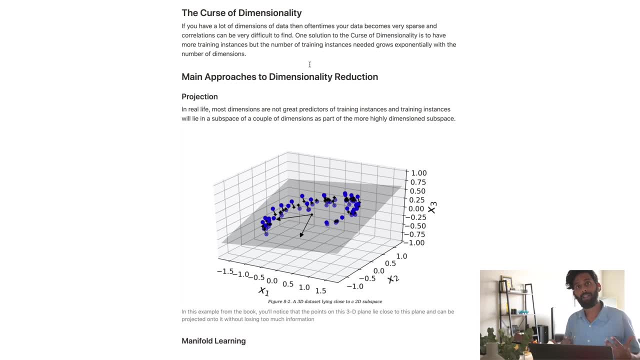 data tends to be sparser as you increase the number of dimensions. What that means is that the actual amount of information that you can actually model on contained per column reduces as you add more and more columns, And so dimensionality reduction tries to find the 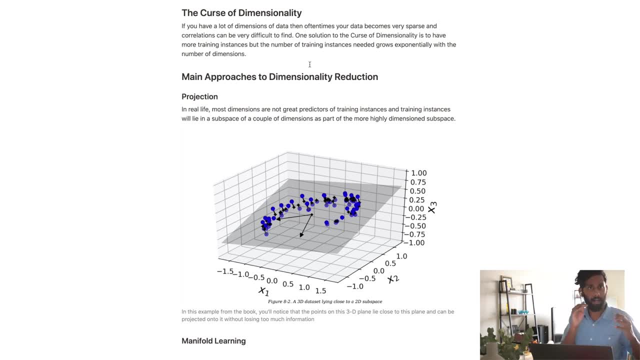 different subspaces in your data that have the most information in that, And we'll get to what subspaces mean in this context in a second. So one solution to the curse of dimensionality is to have more training instances, But the number of training instances we need grows exponentially. 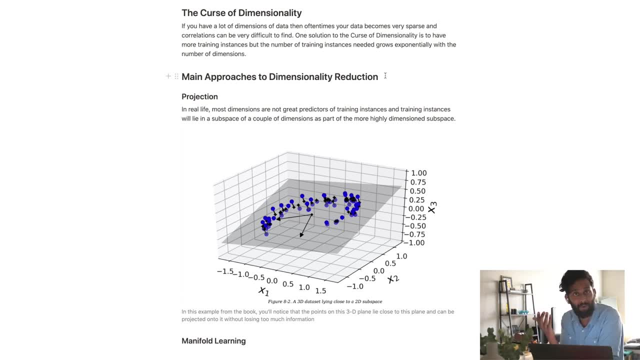 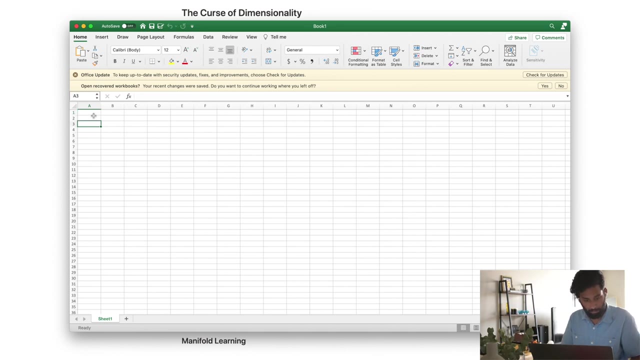 with the number of dimensions, So every time you add in a dimension, for example, right? So imagine I have a data set And actually let me just go ahead and I can even pull up a Excel file right here And let's say we have a feature one. Let's say feature one, feature two and feature three. 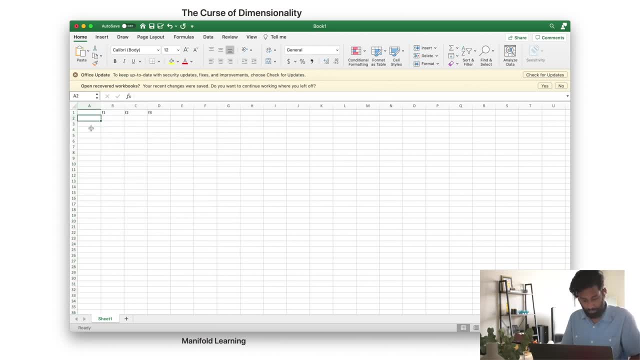 And then let's go ahead and say we have row one, row two, Well, and actually let's just use the Excel column or Excel row numbers to count. You'll notice that if I have, for example, let's say I have- four rows of data, right, So rows two through five, If I was to add another. 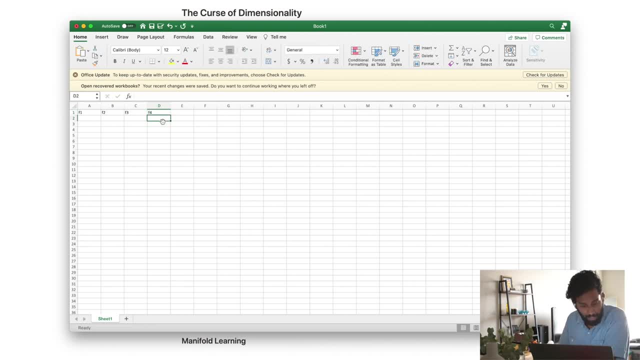 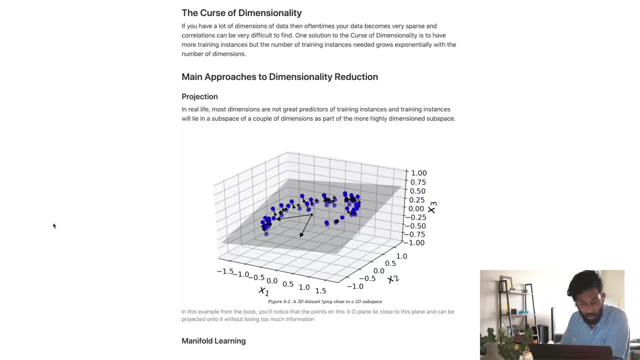 dimension. so if I go F4 over here, then I just added another four records of data. So every time I add a new dimension- or sorry, every time I add a new- either dimension I just add a new dimension Or line of records. I'm adding a tremendously larger amount of data to our data set And then 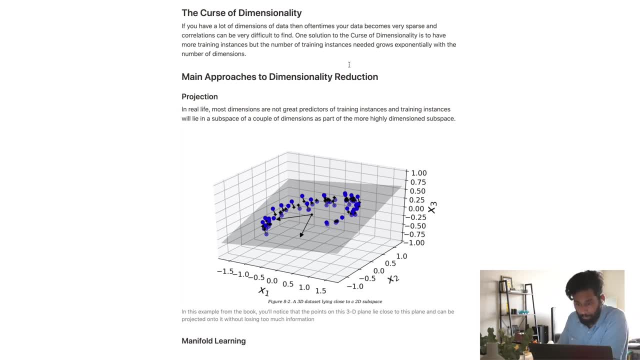 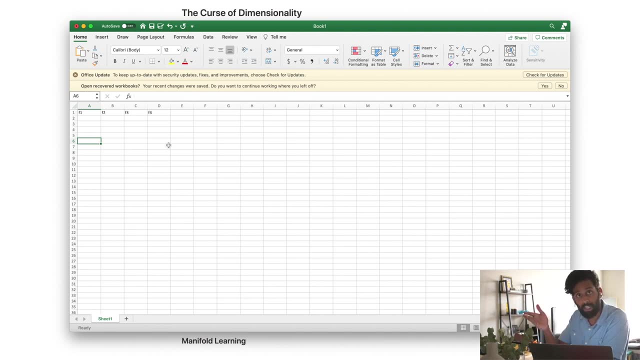 it increases exponentially as time goes on. So, as you can see, if we add a training instance down here, every time we add a dimension, that's just another set of training instances, another column of training instances we need to add. Basically, this could lead to a problem where 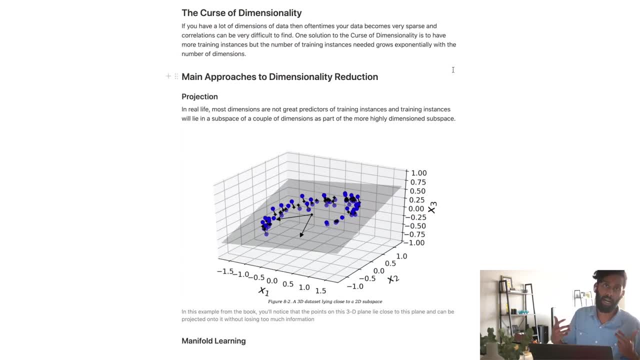 you have way too much data to train on, And that becomes a real issue if you do not have the computational resources in order to handle all that data. So there are a couple of main approaches to this, And I'm going to go ahead and show you a few of them. 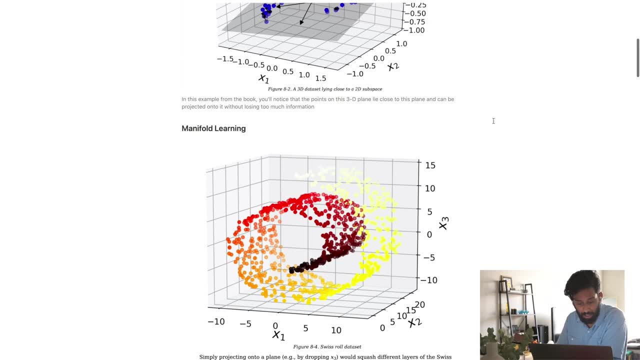 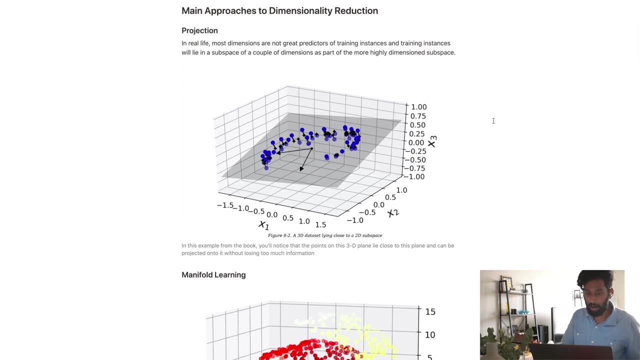 So the first one is towards dimensionality reduction. There's something called projection, There's manifold learning And then we'll go over PCA, the actual ways we handle it. So what projection does is it takes the assumption that in real life most dimensions are not great. 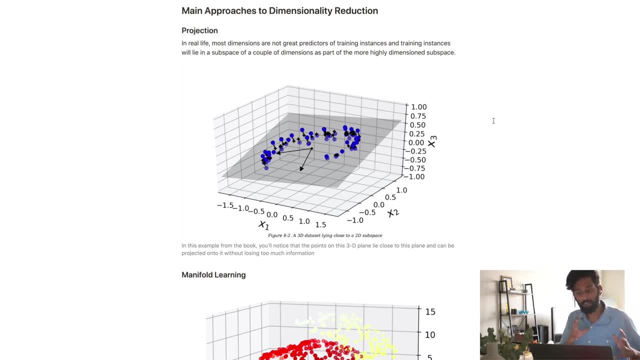 predictors of training instances, And training instances rely within the subspace of a couple of dimensions that are more predictive of anything than anything else. So what do I mean when I say that? Well, let's take a look at this graph over here. You'll see we have a three-dimensional 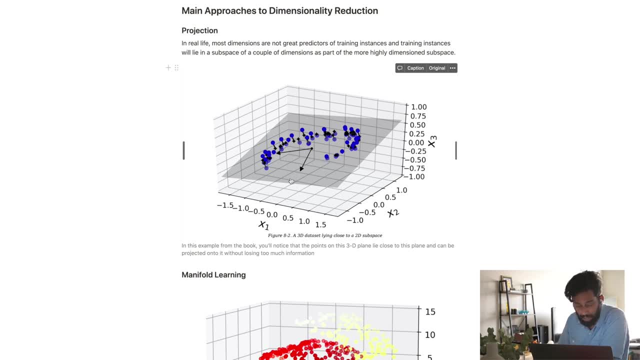 space over here. And what might happen is that we have a three-dimensional space over here, And what might happen is that, even though this is a 3D space, this plane over here contains most of the data. And how do we know that? Well, if we look at the- let's call it- the X3 axis over here. 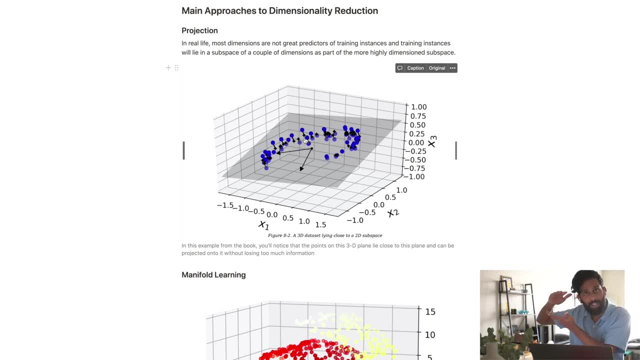 you'll see that the points actually don't have a lot of space in between them, meaning that there may be like one or two unit or 0.25 units away from this plane that we've drawn. And by creating this plane and then plotting every single, like removing the X3 axis and just like 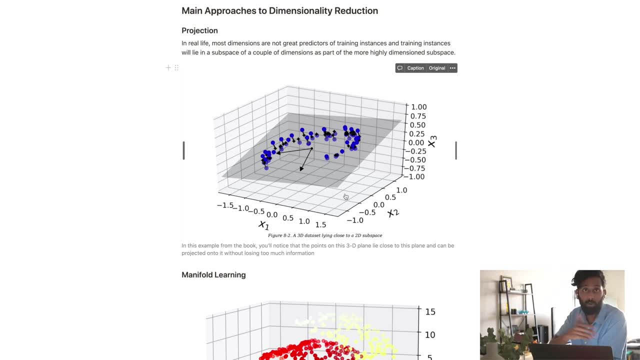 flattening everything onto that plane. we have significant. We have significant. We have removed an entire dimension from our calculations and have not lost a lot of information in the process. And that's the thing about dimensionality reduction: You're always going to lose some. 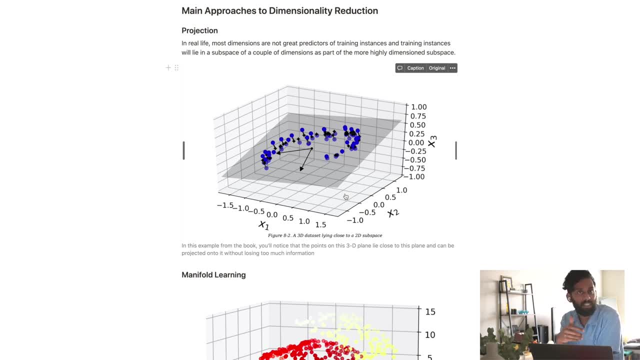 information, but it's all about determining, okay, how much information loss is okay relative to the amount of data I have to process. So that's what we're going to be. That's what we try to minimize. We try to minimize information loss while also minimizing the amount of total data. 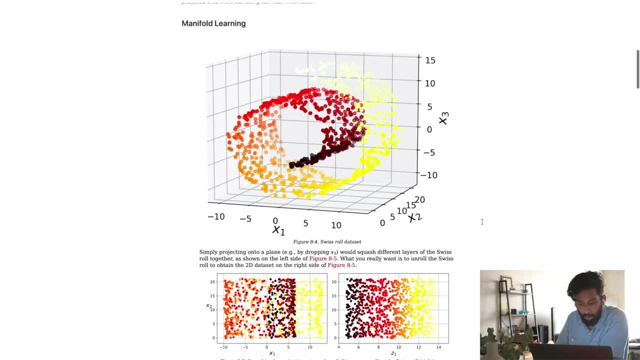 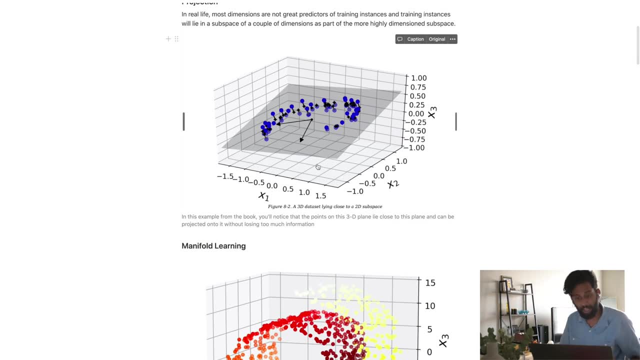 that we have to process Now. another thing you might see is something called manifold learning, And what that means is that it takes into account the idea that maybe you can't draw a plane like this on the data. So this they call it, the Swiss roll data set- is a really common data set to use. 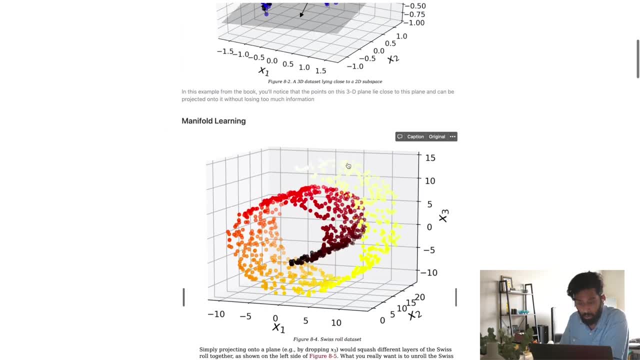 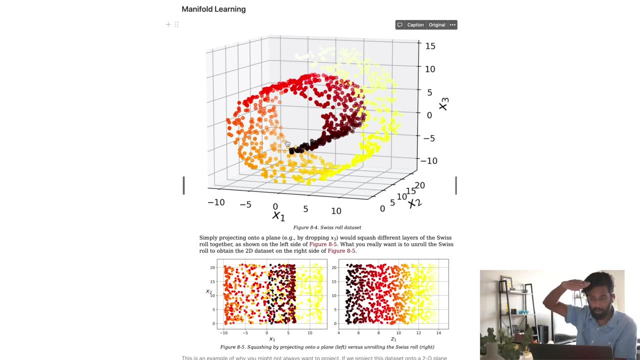 this on If you were to just use manifold or if you were to just use projection, right? So if you look at this graph down here, X1, if you were to take all of the different points and you were to squish them down onto one plane, then you wouldn't be able to separate out the points. And this is. 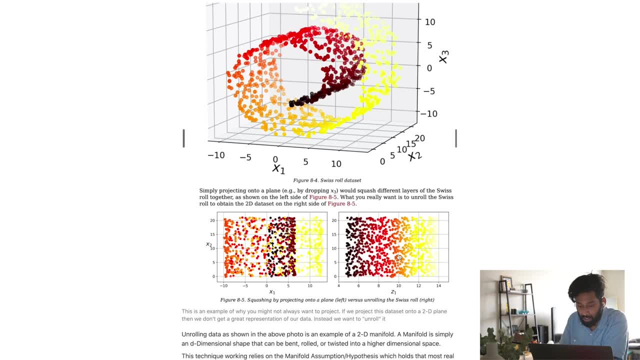 not a great representation of our data Versus. for example, if you were to take a plane and you were to create a manifold- I'll go over what that is in a second- where you have these dark points over here, the red points over here and the yellow points over here, you'll see that this 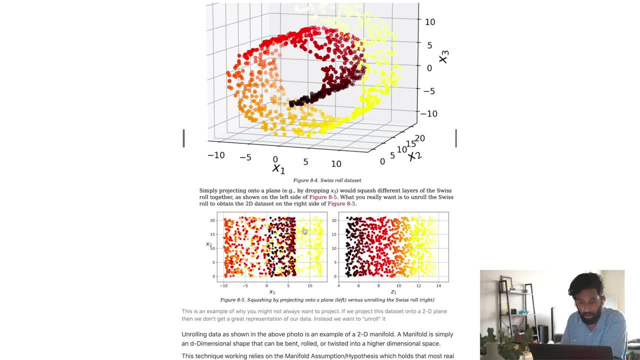 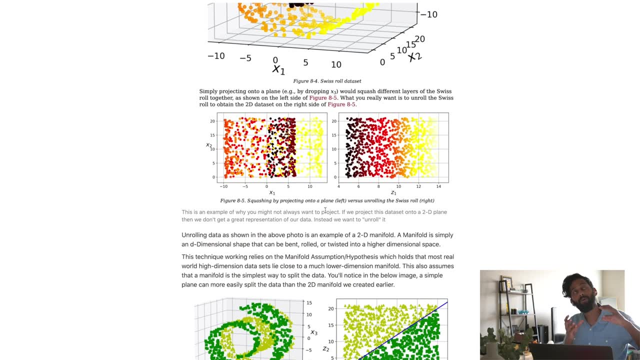 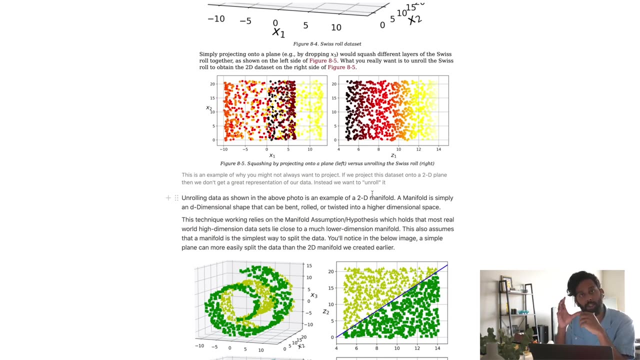 is a much better separation of the data points than you see over here. And what is a manifold? So a manifold is? basically, it is a method. it is when you are able to take a shape of a lower dimension and twist it in a certain way to fit a higher dimension. 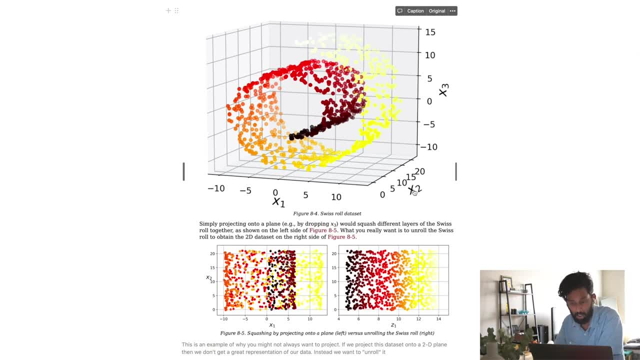 set of data. So what do I mean by that? Okay, so we look at the Swiss roll over here. right, This is a 3D shape. But if I were to take a 2D plane and fit it inside the Swiss roll over here and twist it in such a 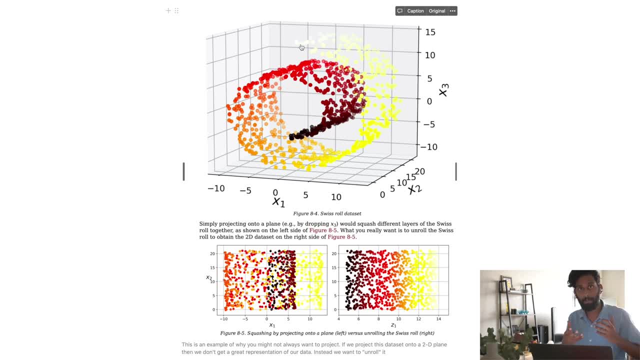 way that it fits inside that Swiss roll. that is a manifold. I've taken a 2D plane and then I've, like, twisted it inside a 3D plane And then, when I project all the points onto that and then flatten it out, I get this over here, which is significantly better than just having a flat plane and then 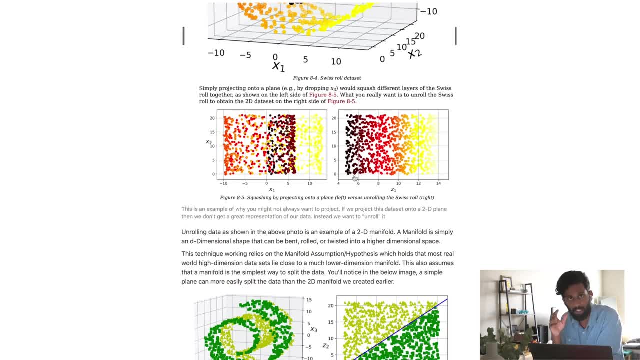 projecting all the points onto it. I highly recommend looking at the chapter here- a chapter- yourself as well, And I recommend that, with all of these videos that I do, you should definitely read the chapter yourself, And the videos I make are kind of just a summary of the content in that. 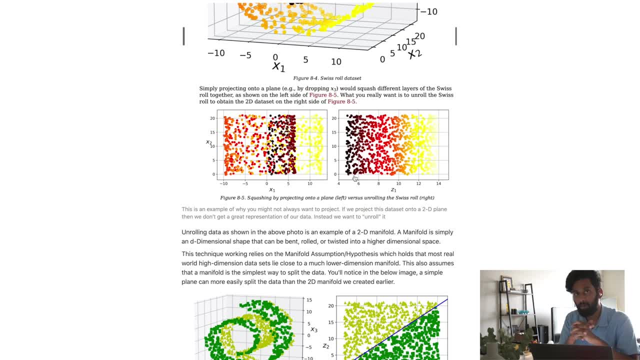 chapter. But I recommend looking at the chapter because if you're not familiar with dimensionality reduction- so much of it is based on this idea of being able to visualize the data in your head- that I think reading over the chapter at least once or twice is very helpful in helping you do. 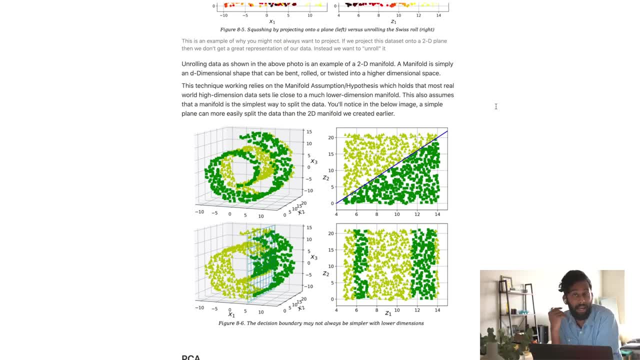 Now, one thing about manifold learning is that this kind of assumes that a manifold is the simplest way to split your data. But if you look at this over here- this figure we have over here again- you'll notice that these green and yellow dots over here are much more easily split by a flat plane. 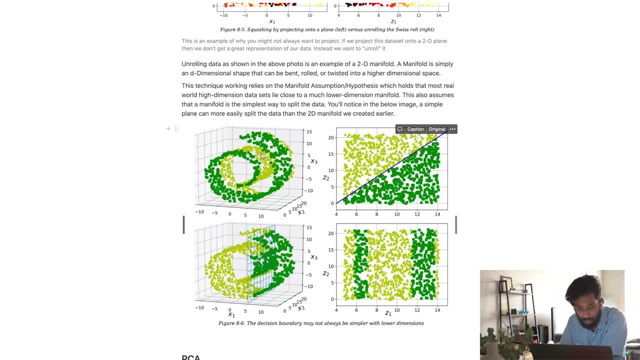 that we just project all of our points onto And if you put that flat plane, you slice it in between that Swiss roll over there, then that's much better than creating a manifold And you'll see that they just put the plane over here, this blue line, versus creating a manifold. Or, for example, 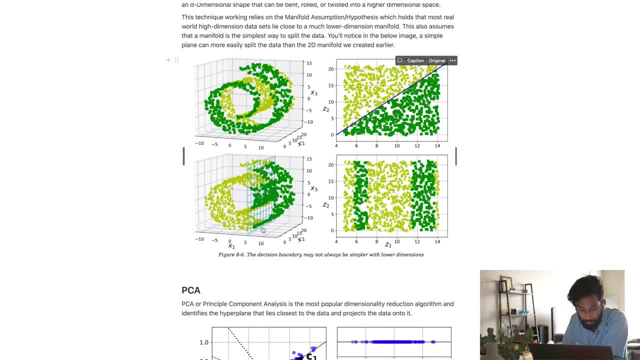 you'll notice that over here all the green points are: anything past x1 equals 5.. That's where you have all your green points And you'll notice that anything past x5 goes in this direction to the right. It makes much more sense for us to use a projection method rather than a manifold method. 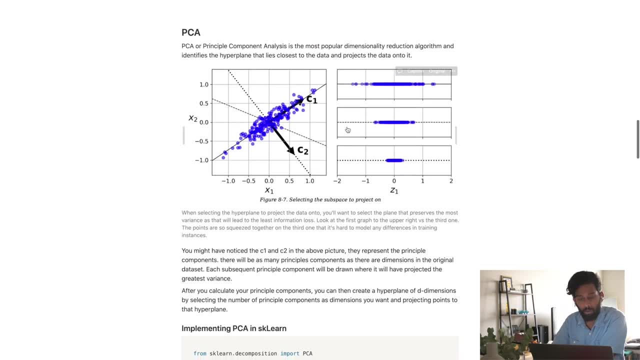 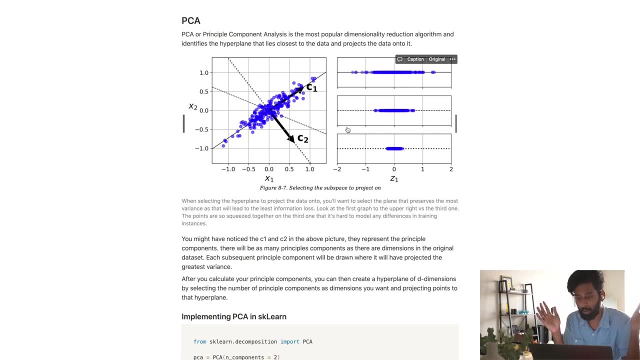 in this instance. So that's kind of the theory behind it. Now let's go ahead and see if we can do some actual application. So principal component analysis is by far the most popular dimensionality reduction algorithm And what it does is that it identifies a hyperplane that lies closest. 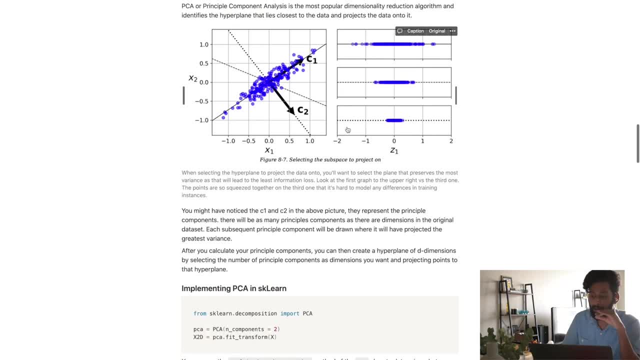 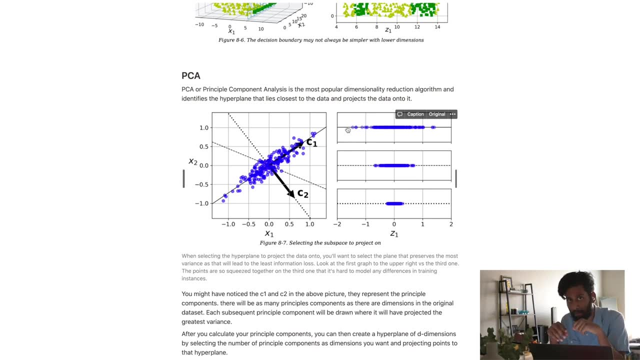 to the data and projects all of the data onto it. And the thing is because we can't really visualize data outside of four dimensions, really three dimensions, but four dimensions- and I'll tell you what I mean when we start coding in a second- but because we can't visualize data. 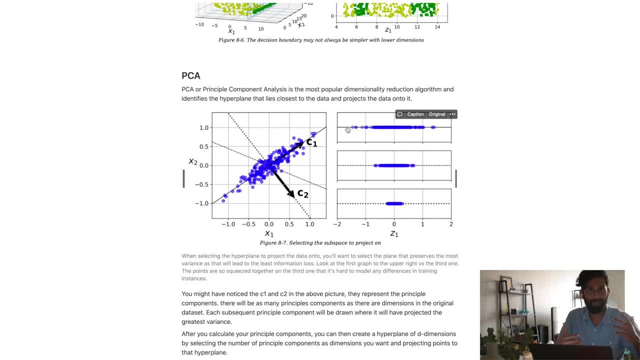 outside of three dimensions. you kind of just have to take the. You have to remember that a computer can not visualize, but a computer can deal with data in an infinite number of dimensions And, honestly, we wouldn't use PCA on 3D data. We would most likely use it on data with 50,, 60,. 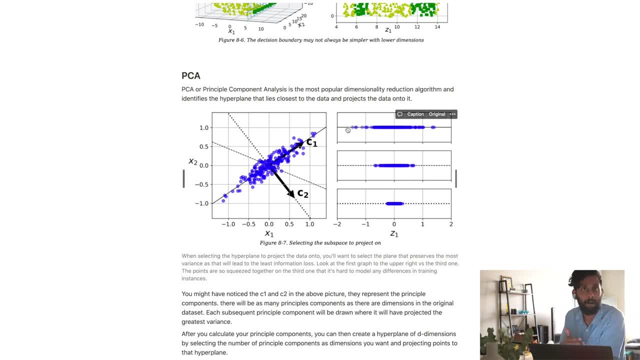 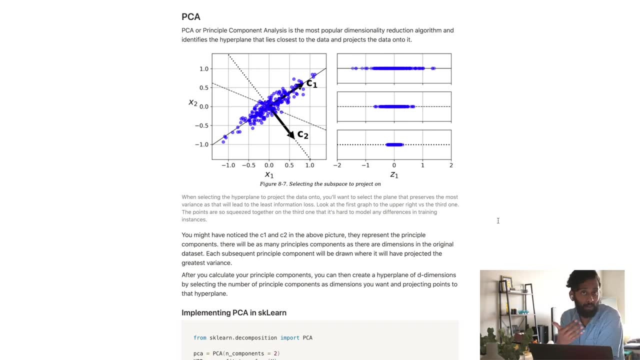 100 columns and data, that's maybe 1,000 dimensions or where n is really high number of dimensions. And the reason for that is because, again, we lose information whenever we add it, whenever we remove dimensions. So you want to reduce dimensions as little as possible. 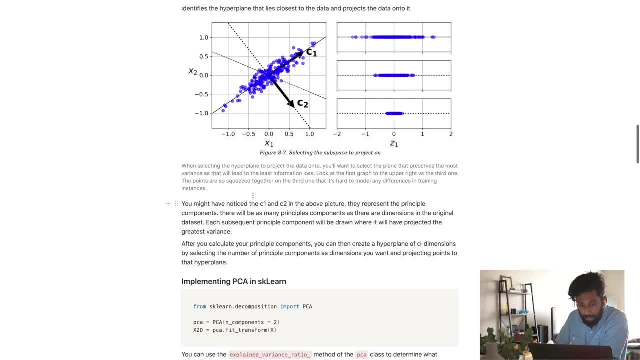 in order to lose the least amount of data possible. So when selecting the hyperplane to project your data onto, you'll want to select a plane that preserves the most variance in the data, because the variance is where your information will lie. So, for example, if we take this data over here, you'll see that there are three different. 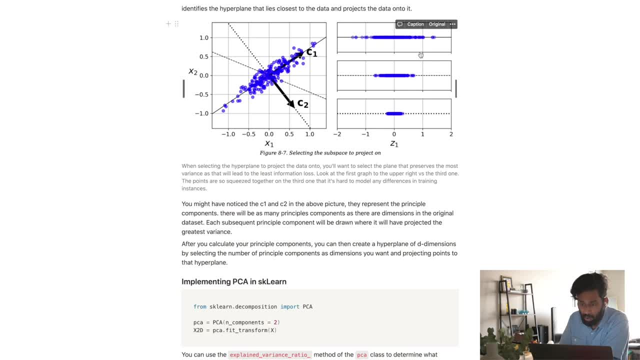 hyperplanes that they picked And I believe C1 is the one we're looking at over here. You want to look at this one, which is this diagonal line over here, because it spreads the data out the most and gives us the most variance, which allows us to actually see the differences in the data. 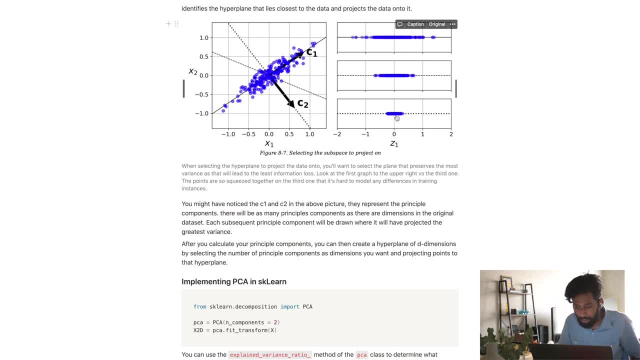 So, for example, imagine we went with this third one over here, which is: this would be, if you had this hyperplane over here, the dark square line one over here. As you can see, there's hardly any difference in the data and I can't really tell what's going. 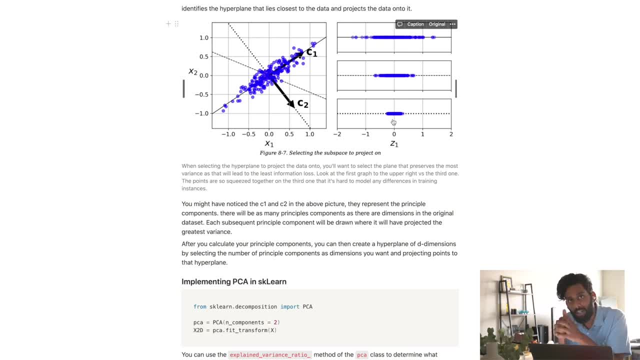 on and what makes the data difference from each other? Because, at the end of the day, if you think about it, what are we trying to do with data analysis? We're trying to find variance And then use that variance in order to obtain information. So, for example, when fraud detection is an amazing application of machine learning and an amazing application of data science, you're not trying to find the person who uses their credit card regularly. You're trying to find the person who uses their credit card irregularly. Basically, where is the variance? 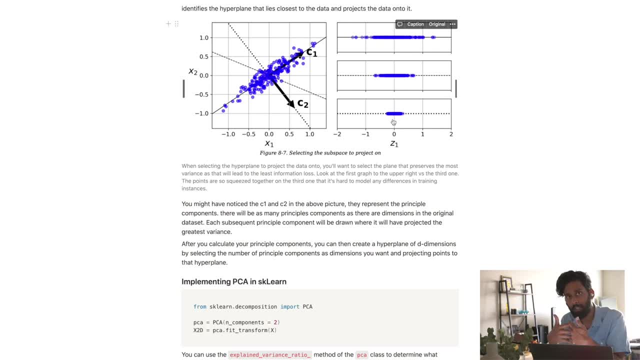 So variance is exactly what we look for in most machine learning applications, And that is why you want to find the hyperplane that gives you the most variance, And in this case, it would be the hyperplane defined by C1, vector C1, over here. 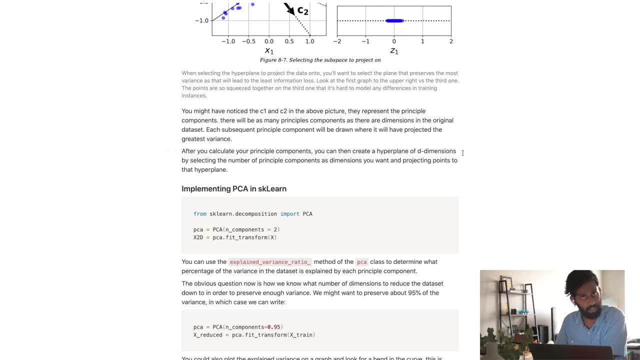 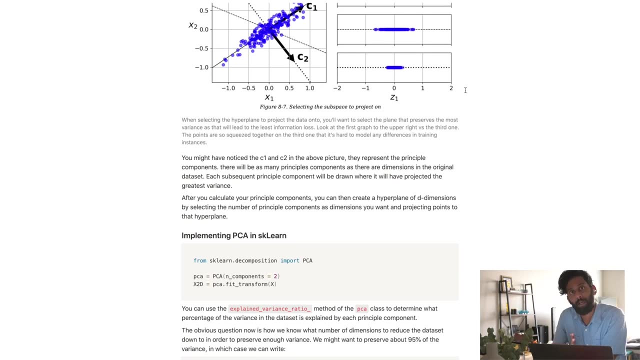 Now why they use vectors. I'm not 100% sure. I think this is where you start getting into linear algebra, which is, at least currently, beyond what I fully understand, But they do use vectors. I just kind of think about it as like: okay, what line can you have that has the most variance in it? 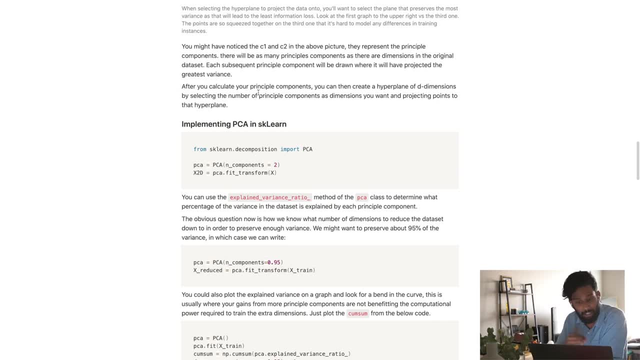 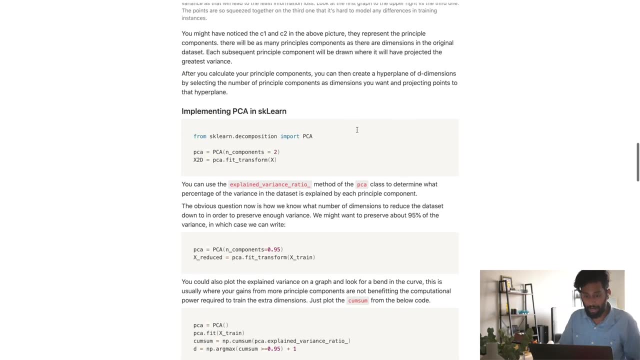 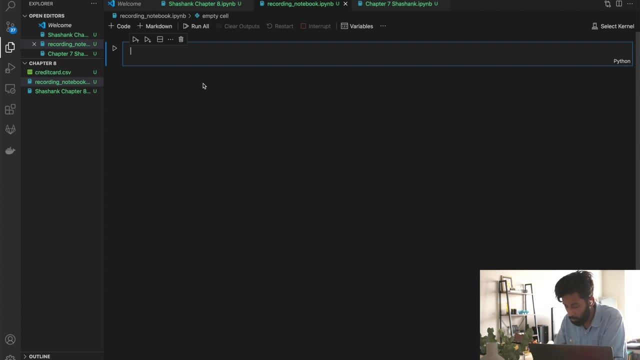 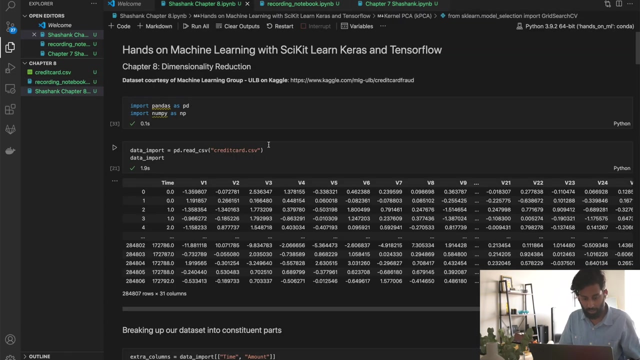 So after you calculate the principal components, you can then create a hyperplane of D dimensions by selecting the number of principal components as dimensions you want and then projecting the points onto that hyperplane. And let's go ahead and just get into the code. So I'm going to open up a Jupyter notebook and we are going to use a specific data set. So this is a credit card data set. 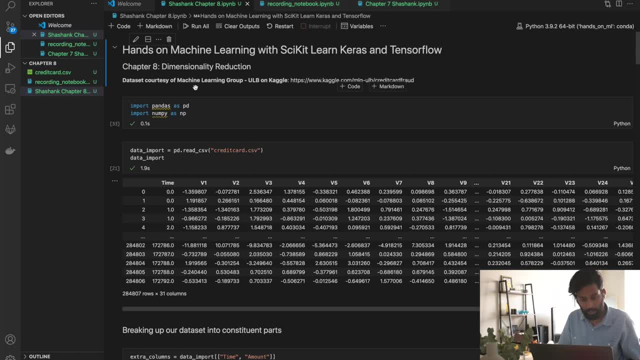 Let me So. this is from the machine learning group And I'm going to type in hyphen ULB on Kaggle, And if you just go to this URL over here, you'll be able to find the data set that I'm using. It's a relatively large data set and it will have enough dimensions for us to actually do some kind of a reasonable PCA on. 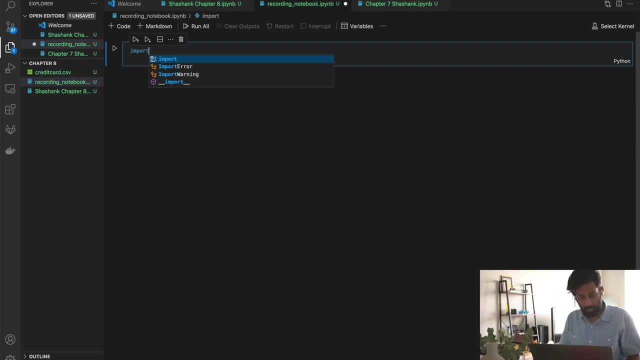 So let's go ahead and do our normal imports first. So let's go ahead and say: import pandas as PD And then import numpy as NP, And then I'm going to run this on my hands on ML, And then I'm going to run this on my hands on environment, and the hands on ML environment just has scikit-learn, plotly, pandas, numpy, you know just your basic stuff over there. 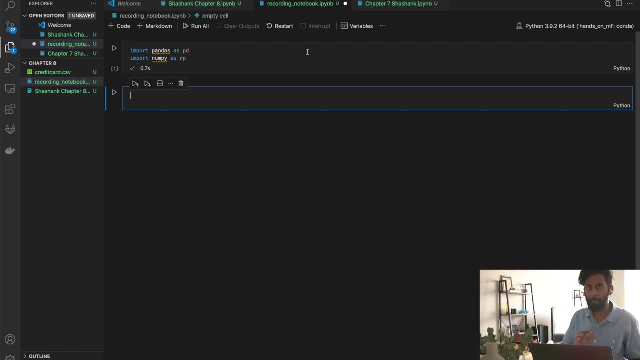 And for those of you that don't know what plotly is, stick around. Plotly is an amazing graphing library inside Python and way better than matplotlib in most cases, And I'll show you why in a second. Get some water, All right. so let's go ahead and import our data. So data underscore import equals PD dot. read CSV: Just reading our CSV. 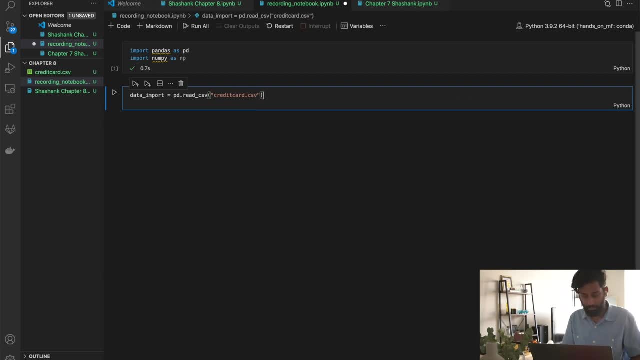 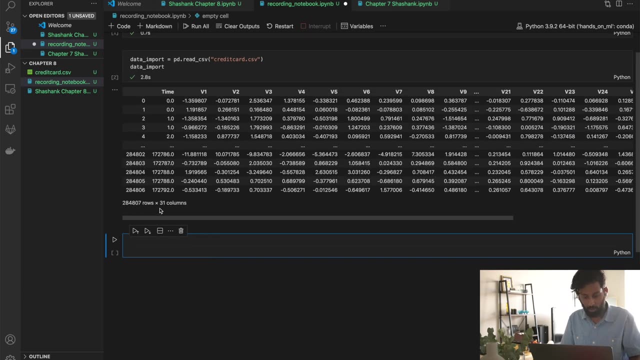 Credit card dot, CSV. And then let's go ahead and take a look at it, So you can see we have a 284,000 rows and 34 columns, So 184,, 1,, 2,, 3 times 31.. 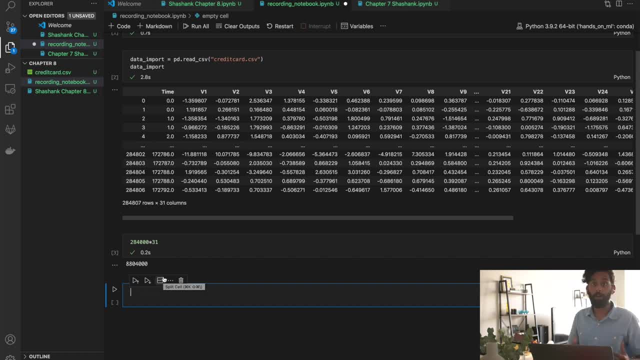 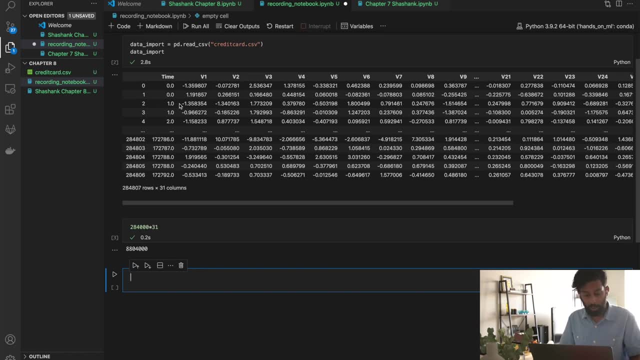 You can see, that is 8.8 million records. So, you know, not an enormous data set, but definitely not a small one. So that's why I wanted to use this one, And I mostly wanted to use this one because of the number of columns that we have. 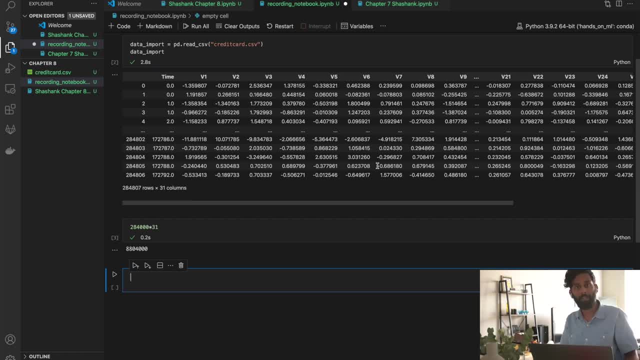 Because 31 columns is a lot of columns to work with, And this is an example of where PCA might be useful. So let's go ahead and get started. So the first thing I want to do is I want to only include these V's over here. 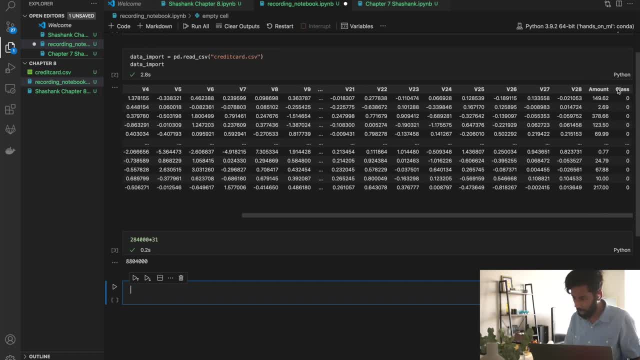 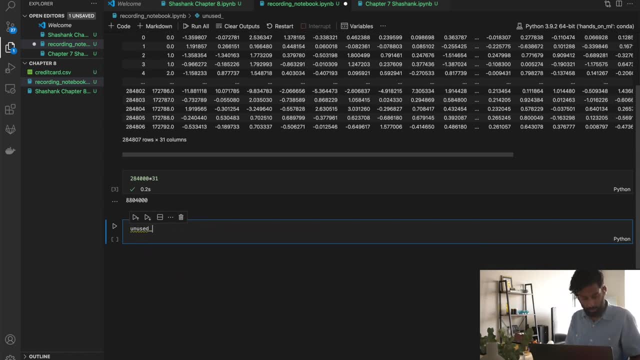 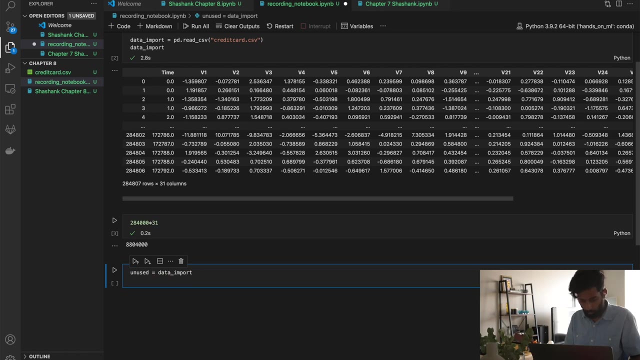 So these V's are basically your features that you care about. Amount and class I don't really care about, and time I don't care about. So let's go ahead and put unused columns And then we'll say that equals data, import, Time and amount. 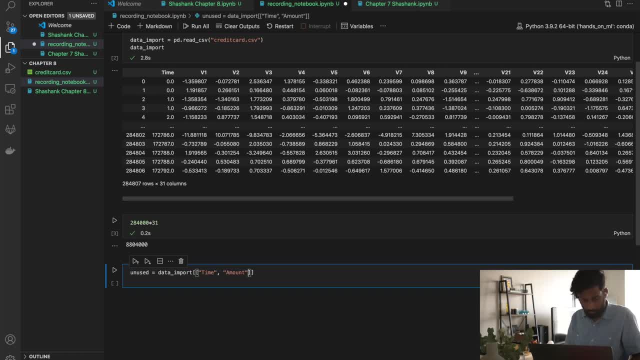 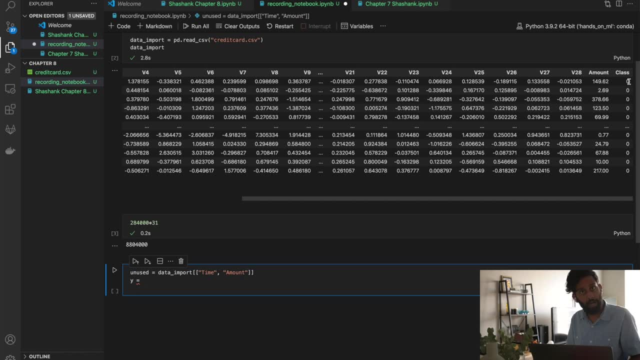 So we're not going to be using that. And then let's go ahead and create our Y, and our Y is going to be: class Zero stands for a non fraudulent transaction and one stands for a fraudulent transaction. So let's go ahead and do Y equals data underscore- import. 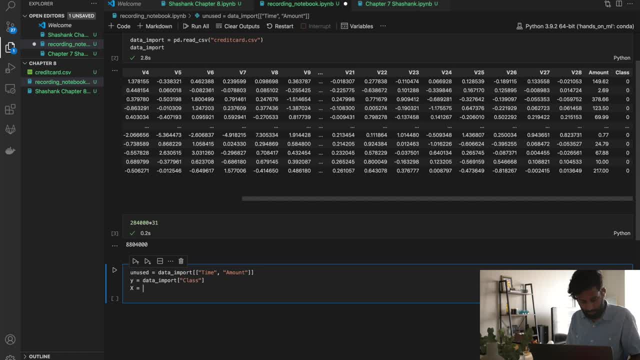 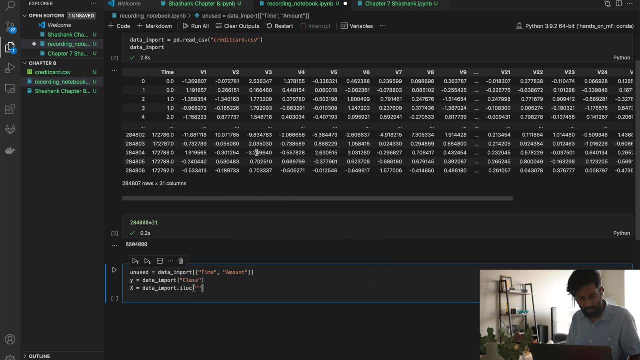 And then we'll say class and then we'll say X equals basically everything else. So data import, dot, iloc. So index is the index locator. I don't know index something. and then we want all of the rows, and then we want columns one through negative two. 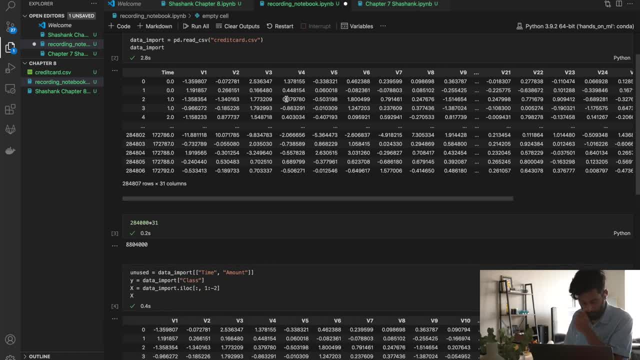 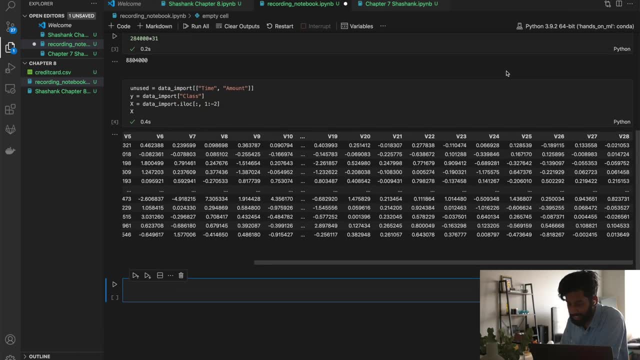 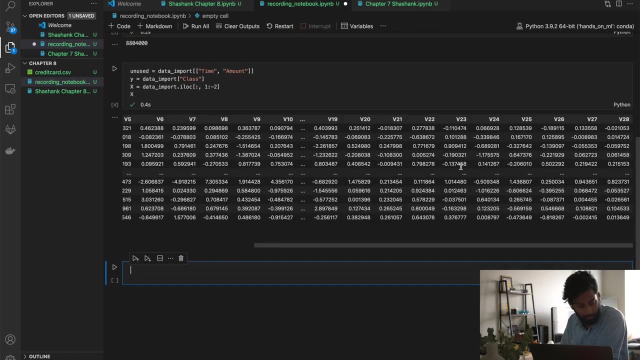 Of course, using negatives, meaning that it starts counting backwards And let's see what we have. So we have data going going, starting from V1 going up to V28.. And that sounds about accurate, Perfect, Perfect. So we've got data tolage as well. 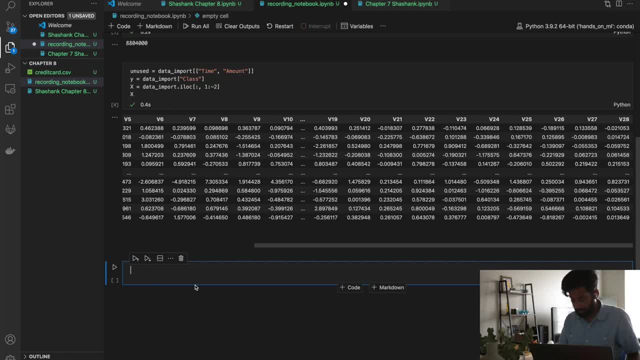 So that we'll just add this: Cool, Alright, so let's go ahead and start doing our PCA. So I am going to start off with a very basic piece of a, So from SKLearnD compilation and import PCA. Alright, so that's our simple import. 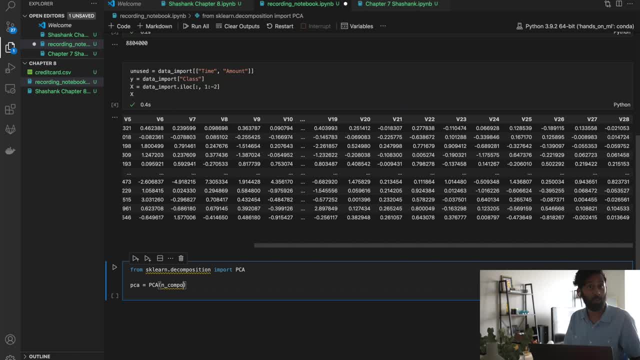 And then we do: PCA equals PCA and components we want to reduce it to. So basically, how many components do we want in our principal component analysis? And I probably should have said it earlier: PCA stands for principal component analysis, So n components equals, let's just say, you know 10.. And then we just do x, 10, d. 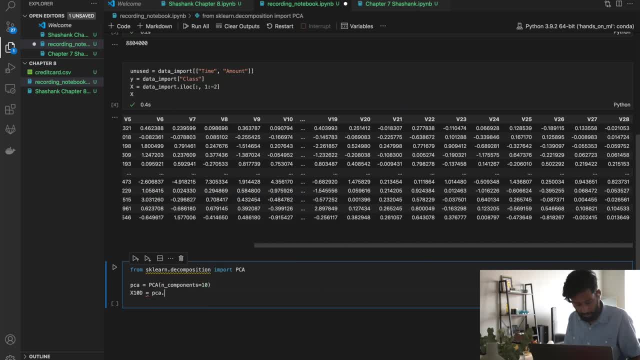 meaning x 10 dimensions equals PCA dot, fit, transform And, as you can see, this falls. this just follows the standard format of all scikit-learn libraries. And then let's see what x 10 d looks like: pd dot. I'm going to turn it back into a data frame because 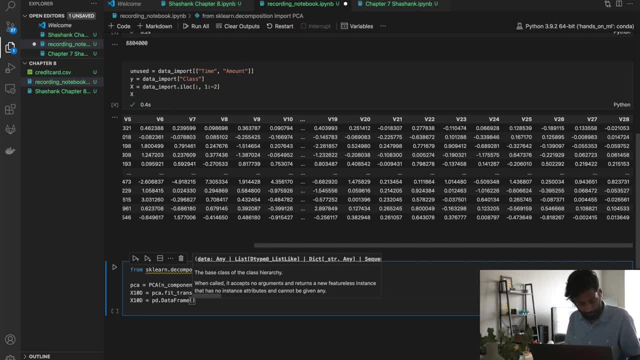 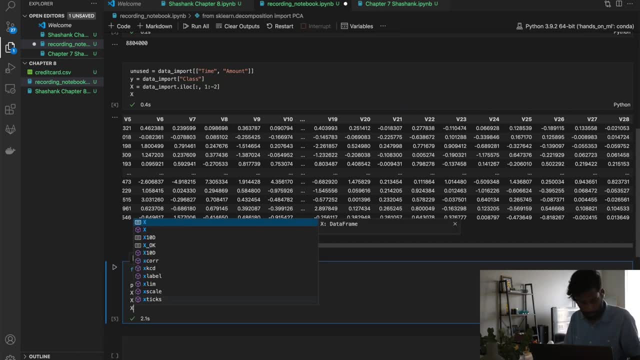 it creates a numpy array. that's super ugly And I want to avoid that. x 10 d And I should probably put x 10 d over here so we can go ahead and take a look at it And, as you can see, we were able to reduce our. 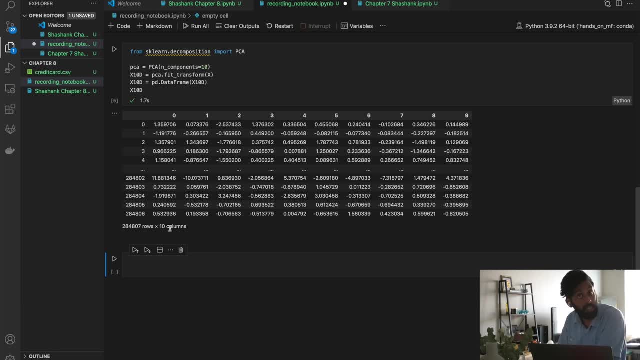 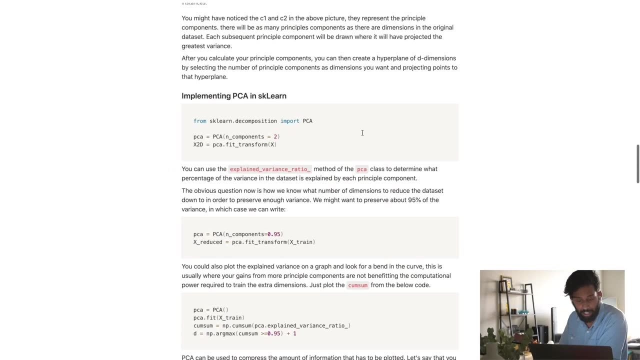 31 columns, or I guess 31 columns, or I guess 31 columns, or I guess 28 columns, down to just 10 columns. Okay, so that was just to show you how easy it is to perform in PCA. Let's go back to the notes and actually start looking at what we did over. 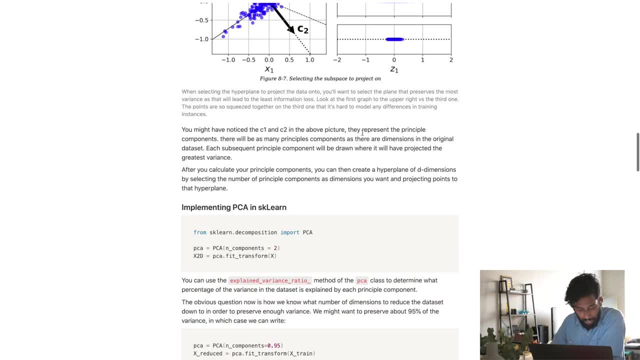 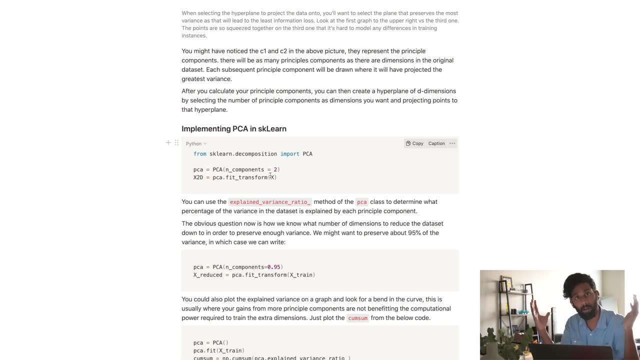 there. So, as you can see, we just went ahead and reduced the amount of data we have from 28 columns down to 10 columns, And there's a couple of questions we might ask ourselves over here. The first one is: okay, how much of the information if we say variance and 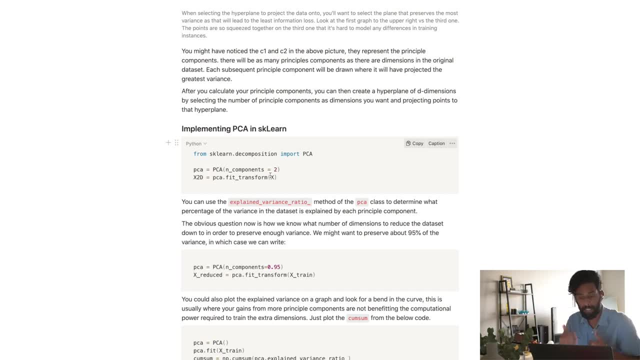 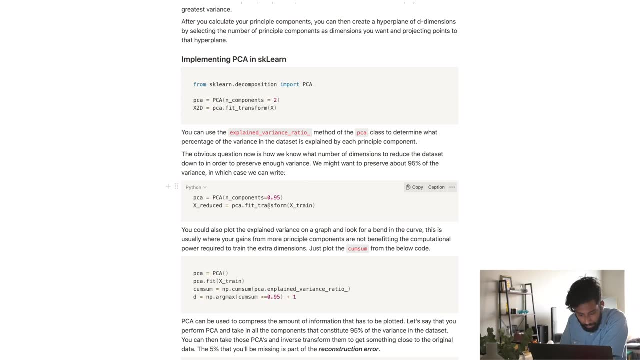 information. how much of the variance have we lost in doing this process? So you can do that by using the explained variance ratio method, or I guess it's, isn't it a method? Oh no, I guess it's a variable. So the explained variance ratio variable will tell you exactly what. 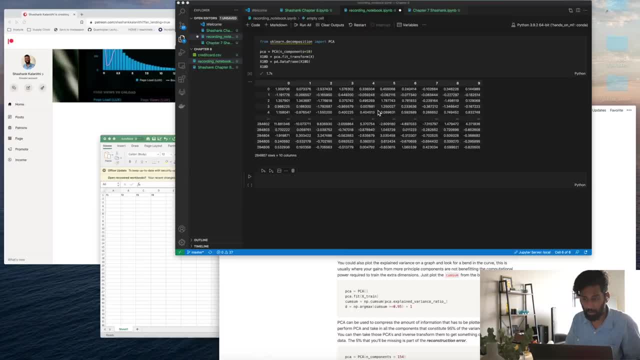 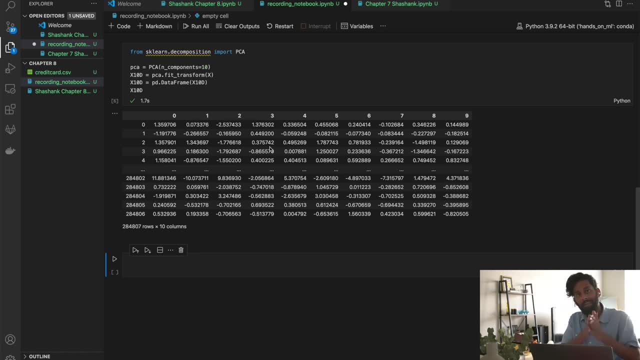 percentage of the variance is explained by each principal component, And one thing I should probably mention is that each the first principal component will have the most information, then the second one, then the third one, then the fourth one, then the fifth one, So each principal. 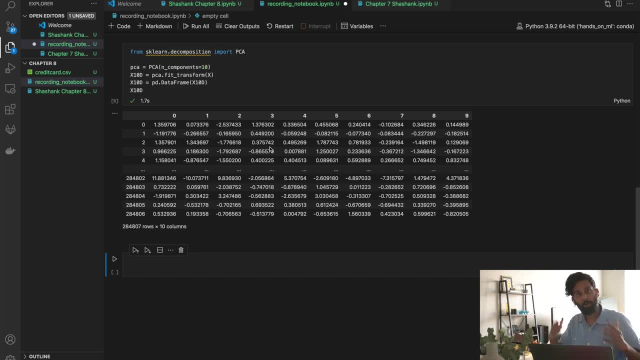 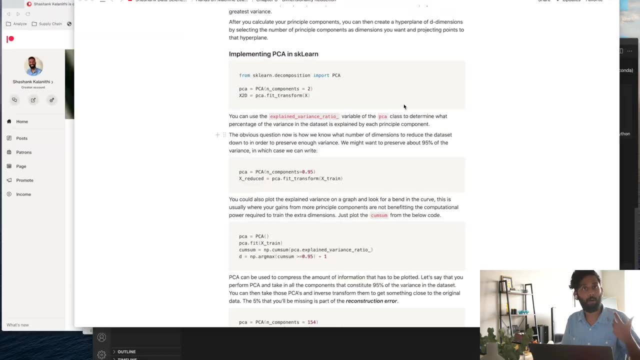 component you have will subsequently have more and more information than the previous one, meaning that the you know first five will have more information than the subsequent five after that. And how do we see how much variance and how or how much information is actually contained? 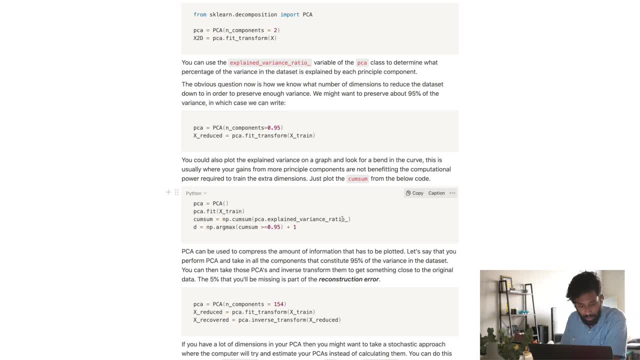 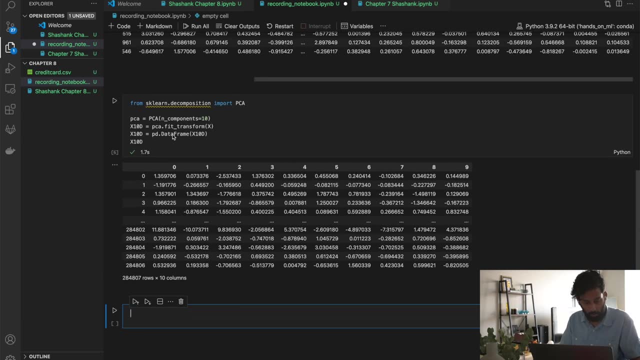 inside these, each of these PCAs. Well, we can go ahead and just run the code over here. So we are going to, let's see, we are going to, let's go ahead and copy this. Oh, whoops, Copy. 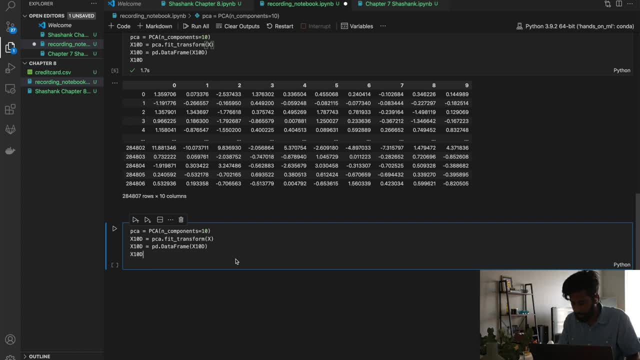 And then we are not going to set this variable over here at all- the number of components- So we're not going to specify the number of components. So I think it should just have the. it'll just have the total number of components that we had earlier. 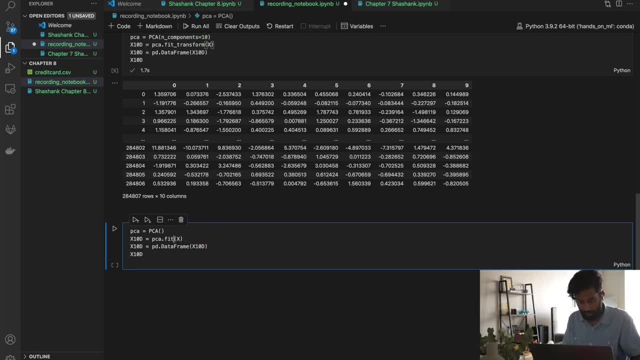 And then I just want to do a regular fit method over here And we'll just call it xd for x dimensions, And then we will do cumulative sum. So the cumulative sum is going to be: the cumulative sum equals npcumulativeSum of pcaexplainVarianceRatio. 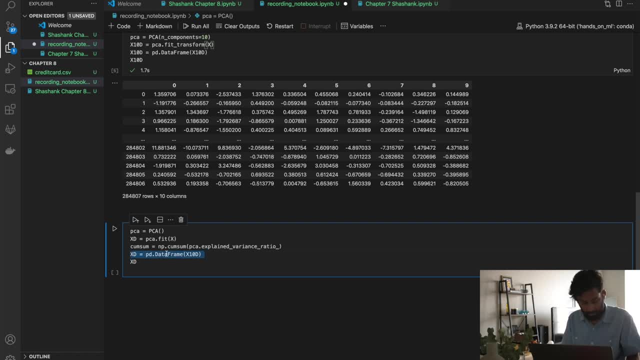 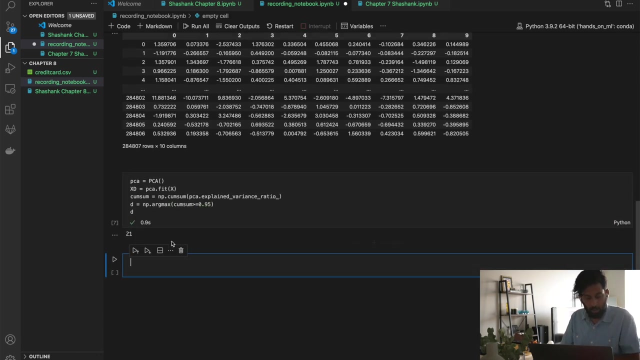 All right, And then d will equal the maximum argument, So npargmax of the cumulative sum that's greater than or equal to 0.95.. So, as you can see what I'm doing over here, right is? I'm asking numpy to tell me. 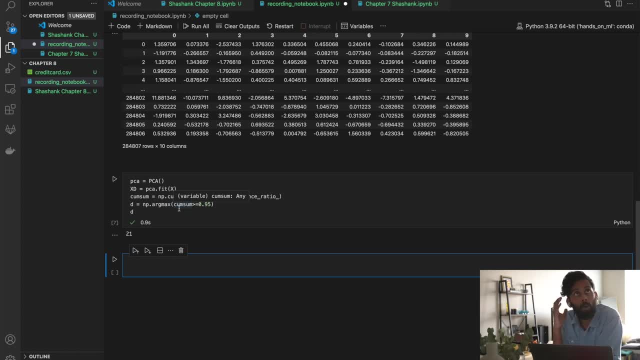 and I'm asking sklearn numpy to tell me: okay, what, how many dimensions do we need in order to explain 95% of the variance in this data? And let me, let me illustrate what I'm talking about over here. So, if you look at, 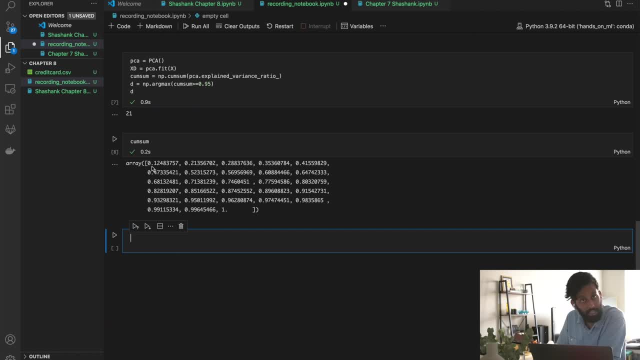 the cumulative sum variable that we created. you'll see that it's a numpy, basically just meaning a list that cumulatively adds from 0 to 1. And each of these represent a. I think this should actually this should have like 28,. 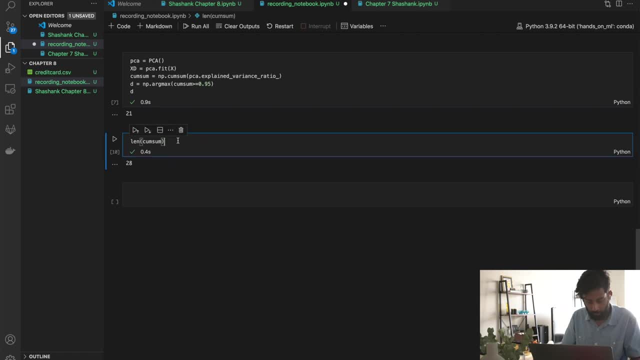 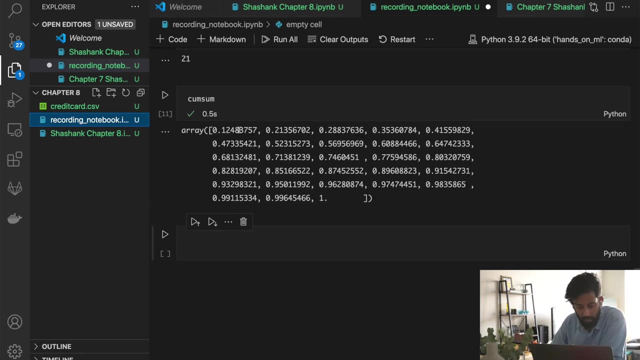 should have 28 items in it. Yep, 28, right there. And let me zoom in for you guys And as you can see over here, what it does for every single column in our data, for every dimension, it tells us how much of the variance in our data. that 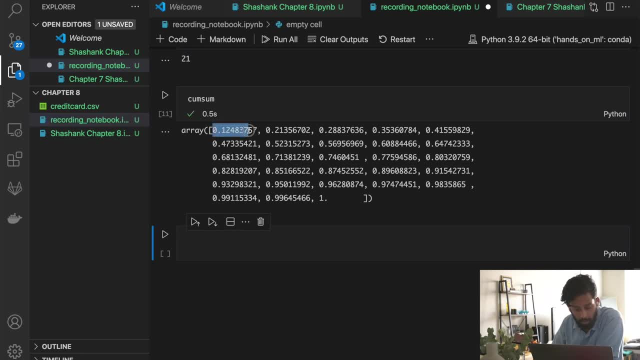 dimension explained. so, for example, the first dimension explains 12.48 percent of our variance, and then the next one plus the first one, because we did cumulative, so remember- explains 21, so that would be about a nine percent difference. so, for example, the first component, the first variable, 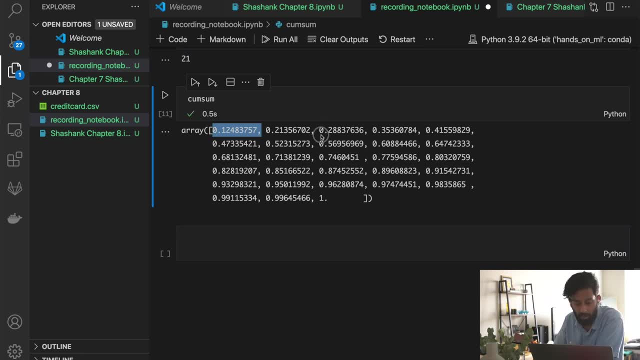 or the first component we have, explains three percent more of the difference than the next variable explains, and so on and so forth. you can see the one half that only explains about seven, and then it's about um, a little bit less than that, and then it's about six, and it goes on from: 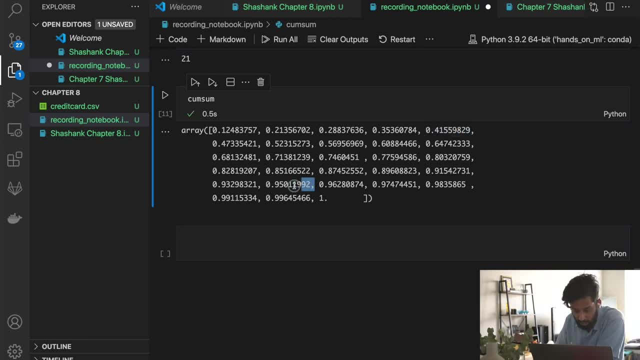 there and we have to go until the 21st component, which is like right here, i believe, before we are able to explain 95 of the variance. what this means is that, again, depending on how precise and how much computation, how precise you have to be and how much computational power you have access, 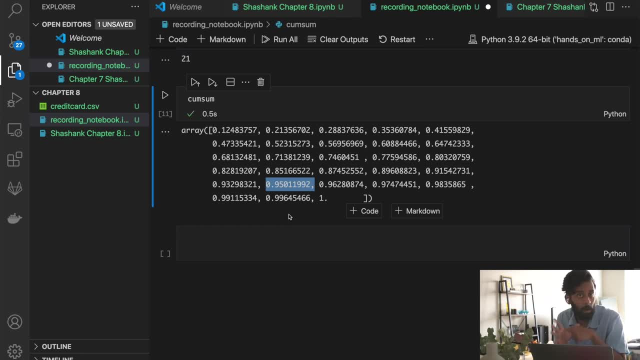 to. you could probably drop the last seven columns of data and just reduce it to 21 principal components and still main and still train a machine learning algorithm. that's just as good as if you had kept all the data. now again, we only have 31 columns. 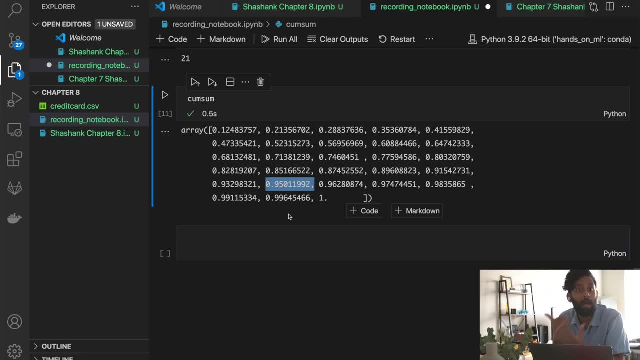 over here and i have a relatively powerful computer, so you're uh, this would not be a example of a uh, of a time in which we would actually use pca, but this is just to illustrate. hey, this is a good good, this is how you would use it and this is one way we determine how many. 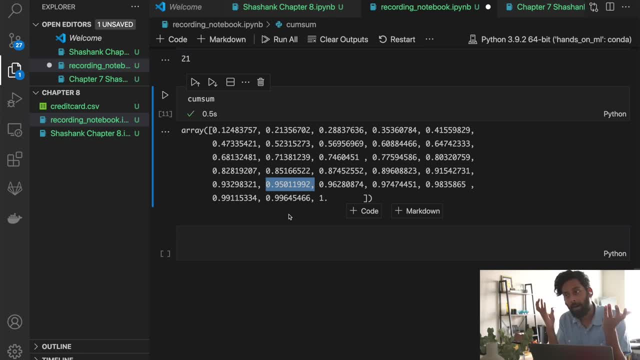 dimensions do we want to keep now? how do you know how many uh or what percentage of the variation you want to keep now? that's up to you, and that's kind of this is where data science becomes more of an art than science, and this is why people hire data scientists. they don't hire data scientists. 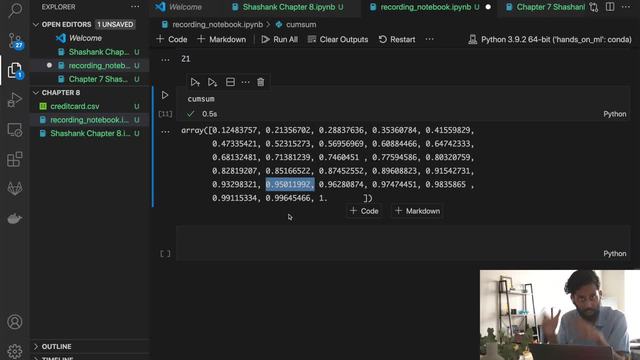 in order to write sklearnimport xyz, like the actual machine learning part, takes like five lines of code. it's all the experience that you put together and all the experience that you generate that is able to say like okay, based on my experience in this industry, for the application. 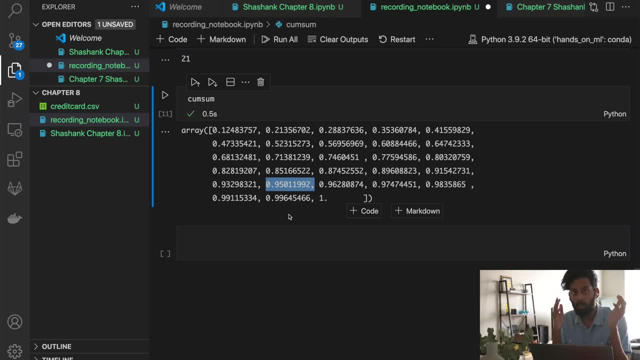 that we want to do so. for example, if you want to detect tumors versus if you want to predict consumer spend at a retail age at a retail company, um, you would have two very different metrics as far as like, okay, what is the level of certainty i need? so, for example, with: 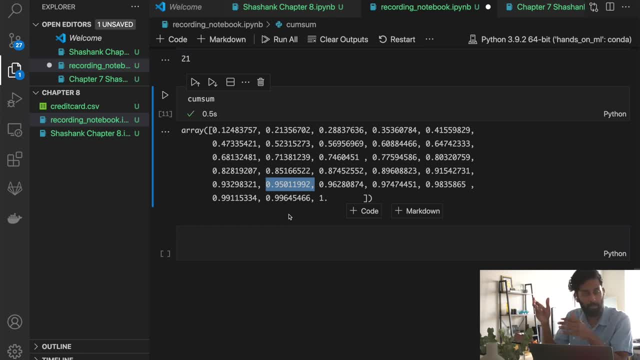 uh, if you're trying to predict tumors inside, uh, they have machine learning learning algorithms these days, specifically deep learning networks, that are able to look at um x-rays or i think it's mris of people and like say, okay, this person has a tumor, this person doesn't, with more. 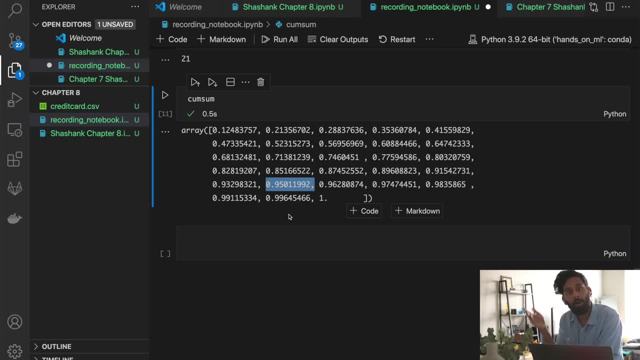 accuracy than most doctors can. um, you might actually want to have an algorithm like that, biased towards a false positive. uh, because you want to be you're. it's better safe than sorry in those cases for most people, versus if you're working retail and you're trying to like you know. 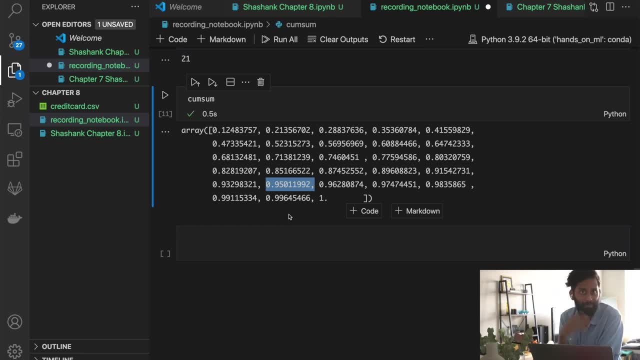 predict consumer spend. you may not want to over predict consumer spend, and the variances you have over there are going to be significantly different, and that's what you need a data scientist for. you know, as you start implementing the stuff, you'll start to see the patterns in it. 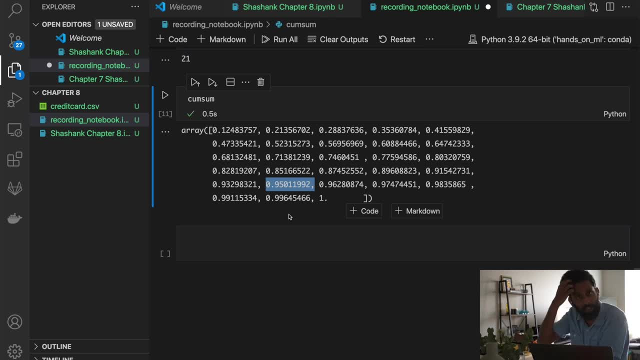 and you'll start to see, like, okay, it makes more sense for me to have this kind of variance over here, but not this variance over there, and so on and so forth. so you could pick 95, for example. right, another method is using. another method you could use is something called the elbow. 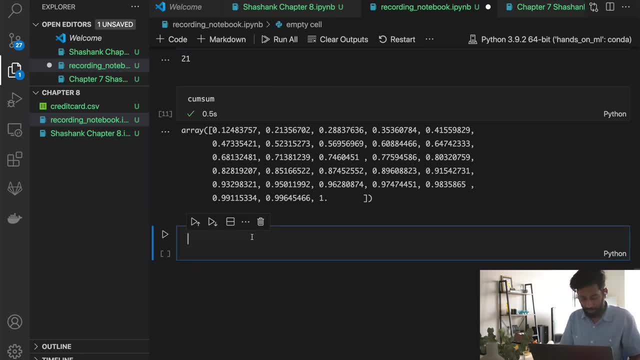 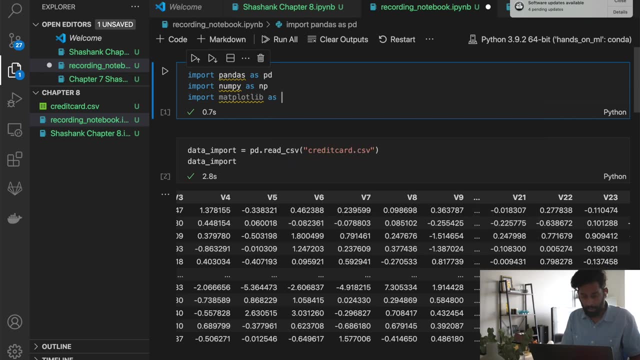 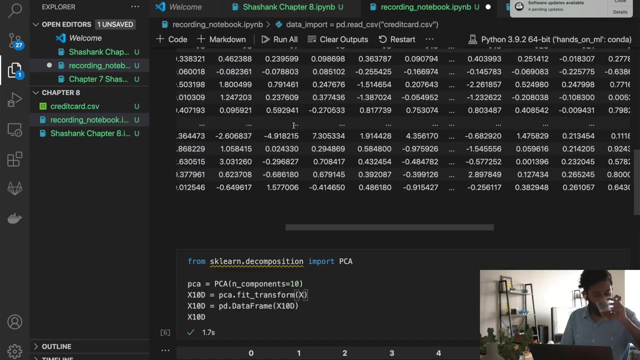 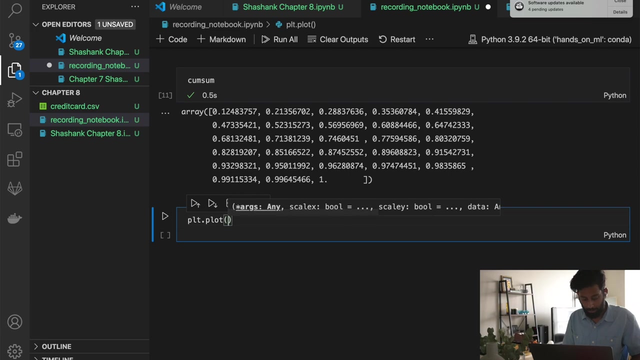 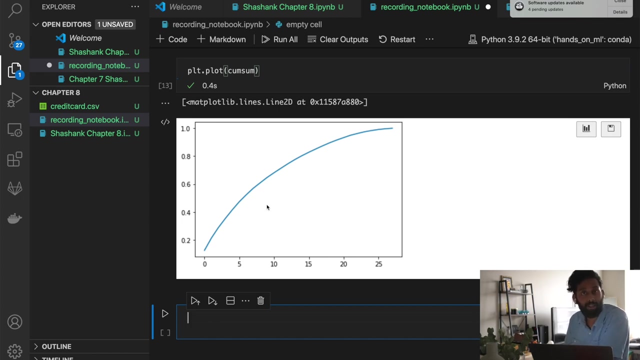 method which we went over in an earlier video, where basically what i do is: let me go ahead and import matplotlib and i'll show you import matplotlib. uh, i can go ahead and plot this. so plotplot equals cumulative sum and what happens is i'm looking for a sharp elbow, after which i would say like okay, after here it's. 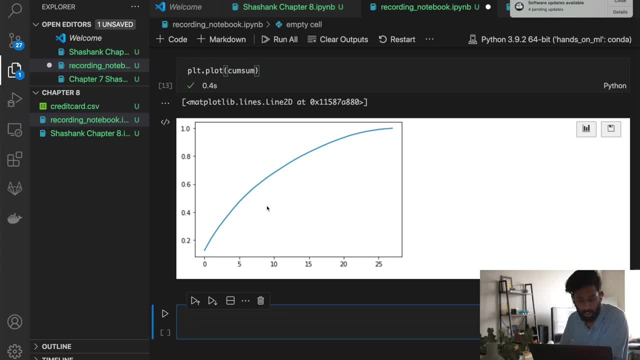 diminishing returns and we might as well, just like, have our principal components up until here. so you'll see, in this data we don't really have a sharp elbow. i'd say like the elbow is probably somewhere like over here, um, but i'm going to go ahead and import matplotlib over here and i'm going 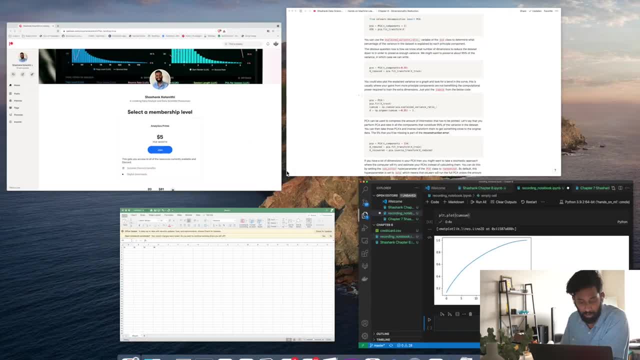 to just give it a little bit more time, because i'm going to go ahead and import matplotlib over here, and i'm going to just go ahead and import matplotlib over here and i'm going to just give it a little bit more time, because it does obviously taper off at one point, at 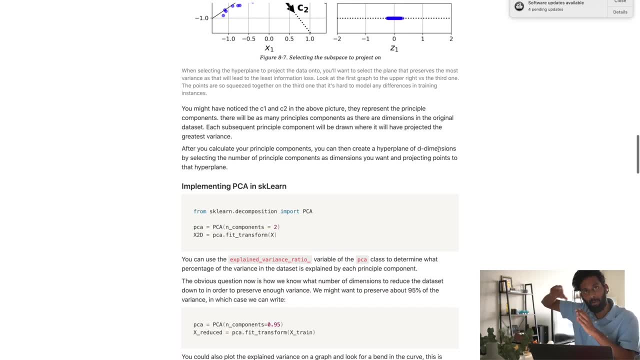 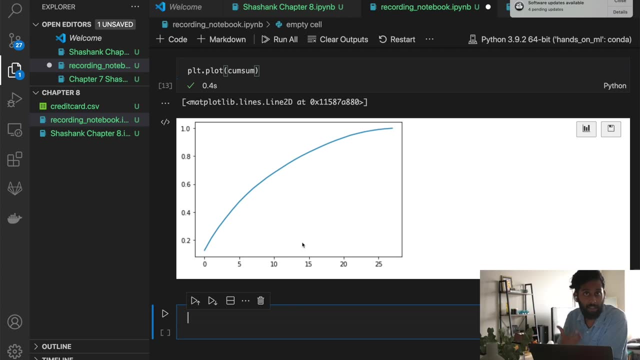 times like your elbows kind of over here, but in the example they're given the book you'll see. oh, i guess i didn't take a screenshot of that, but there's an example in the book where, like, the elbow is like a lot more obvious, and so that's where you might want to use the elbow method. so 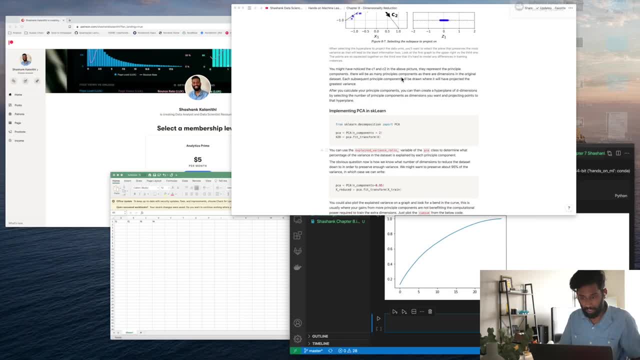 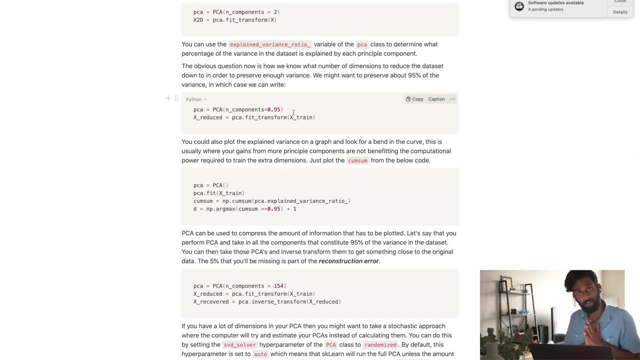 you can either specify the amount, the number of or the amount of variants you want to have, or you can just say album after. we're going to do it that way. all right, let's go to the next section. Say you, for example, wanted to have the PCA algorithm automatically pick the number of PCAs for 95% accuracy or 95% variance. 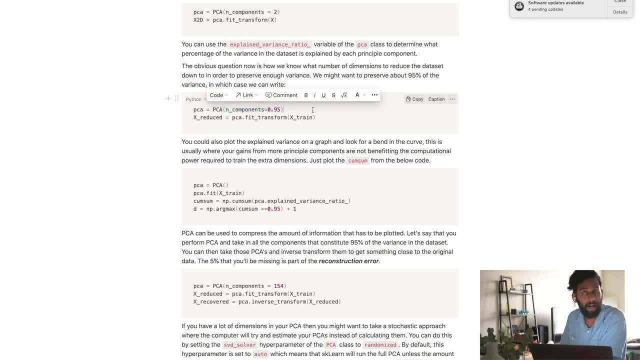 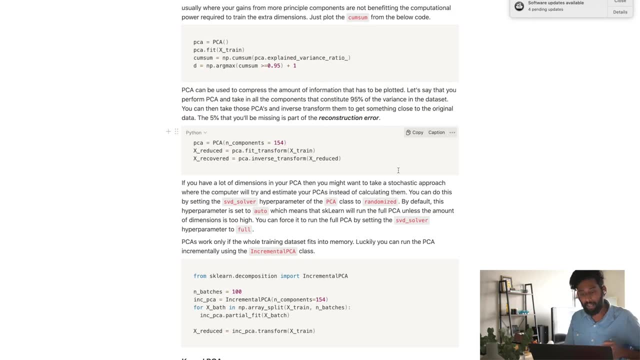 Just tell n components to equal something between 0 and 1, and that percentage is what it'll try and match. All right, So PCA can be used to actually compress the amount of information that has to be plotted or has to be dealt with in your machine learning algorithm. 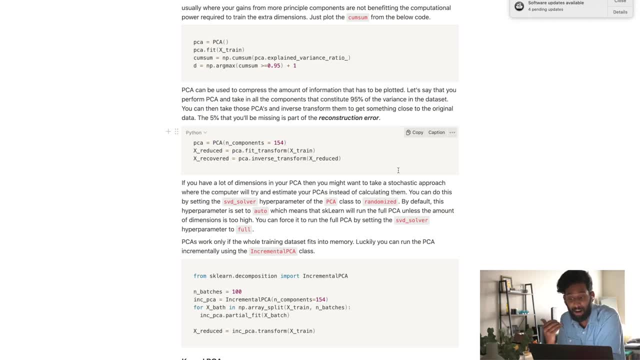 And let's say you perform PCA and you take in all the components that constitute 95% of the variance in the data set. You can then take all of those PCAs and then inverse transform them like you can with a lot of machine learning algorithms or like you can with a lot of the preprocessing steps in SKLearn. 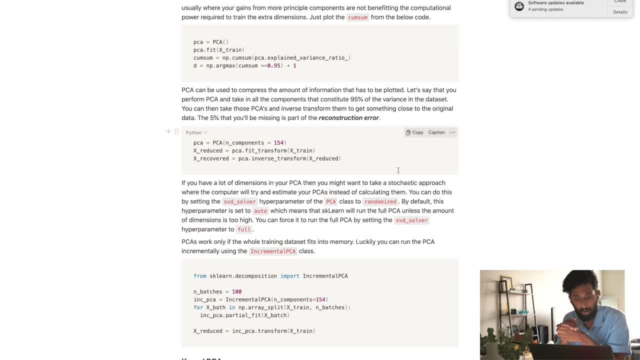 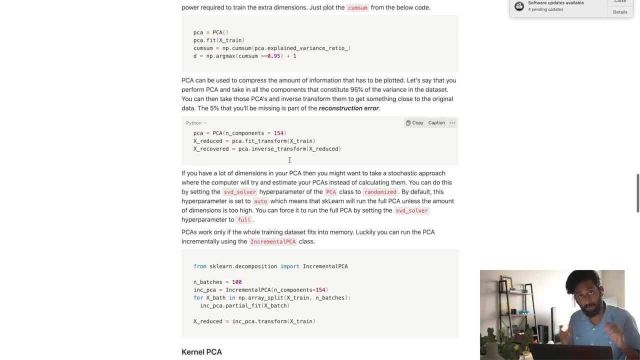 You can inverse transform them and get something close to the original data, Of course, the 5% that you'll be missing. that error is called the reconstruction error, And you can go ahead and inverse transform your data just by using the inverse transform method. 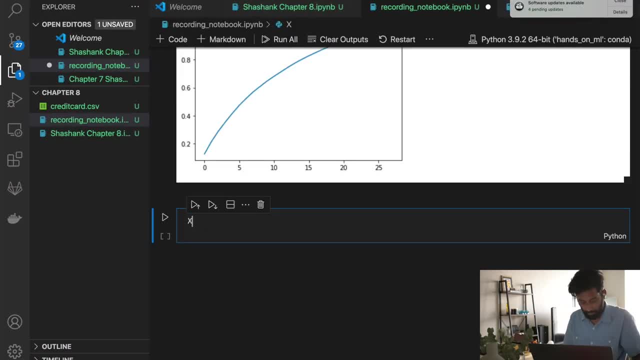 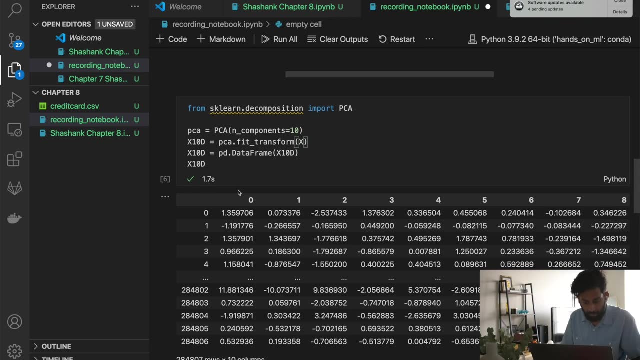 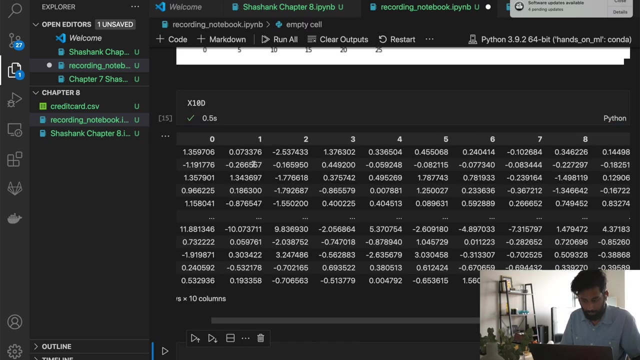 So if I go over here to, I think it's like xd. Oh, did I? Okay, let's just say this: x10d, So x10d. Okay, cool, You'll see, we have our 10 dimensions over here. 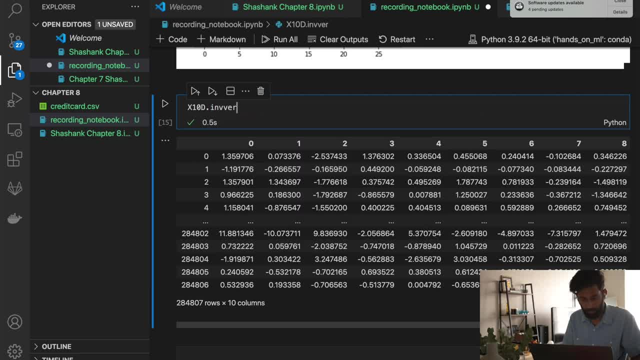 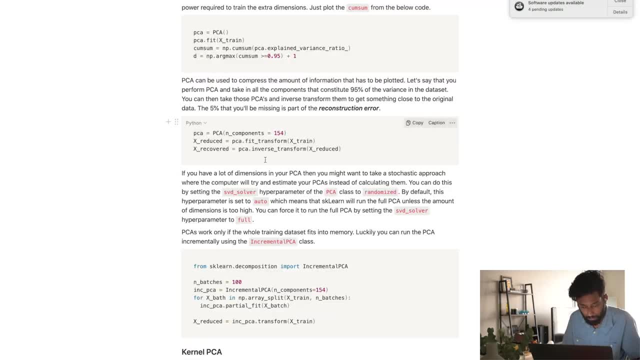 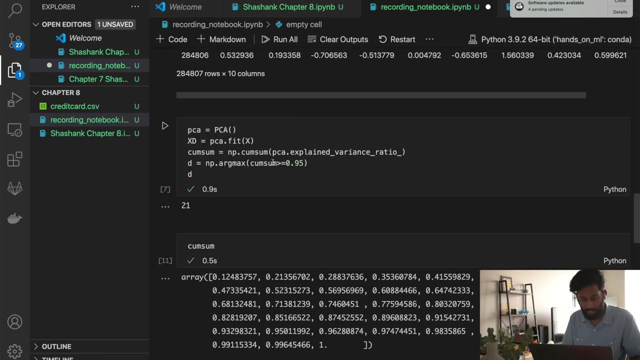 I can go ahead and do an inverse transform- Inverse underscore transform- Wait, can I do it? I don't like that. Oh, PCAinverse transform- Whoops. So what I actually have to do is I have to use the same PCA argument. 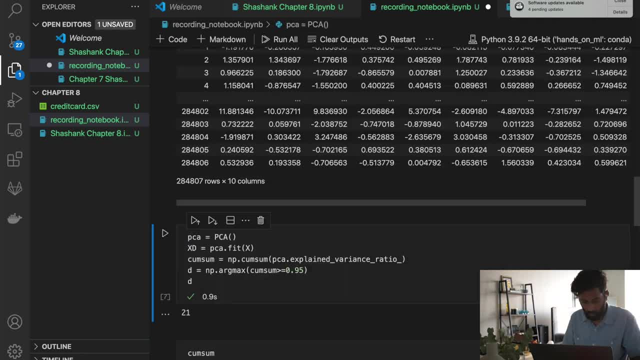 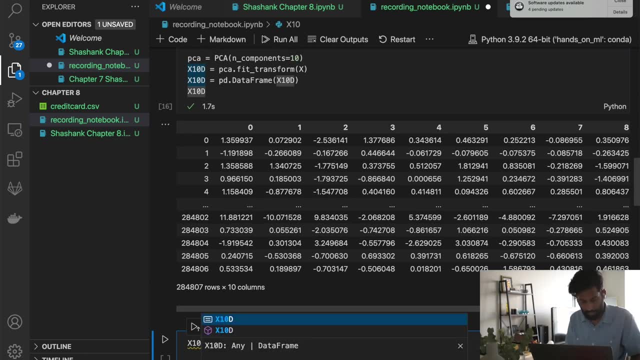 So let's go over here back to our 10d example. Let's run it one more time And then let's do x10d Or, sorry, x inverse, We'll call it that- Equals PCAinverse. transform rx. 10d data. 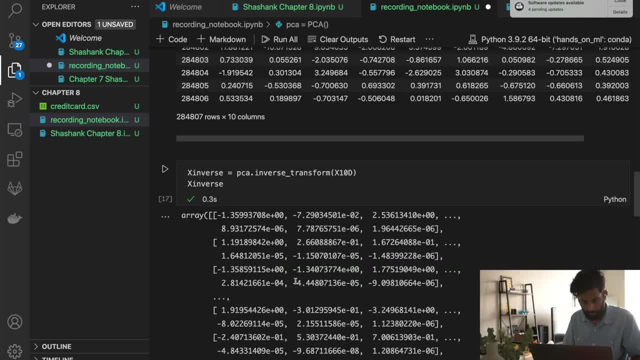 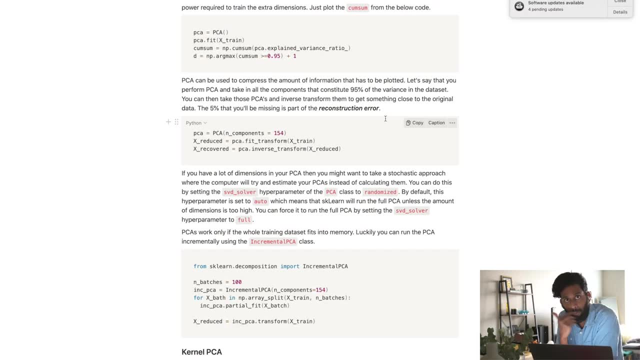 And then we get x inverse And you can see it inverse, transformed your data, And whatever you lose is called your reconstruction error. So that's actually another method by which you can determine how many PCAs you want, how many principal components you want. 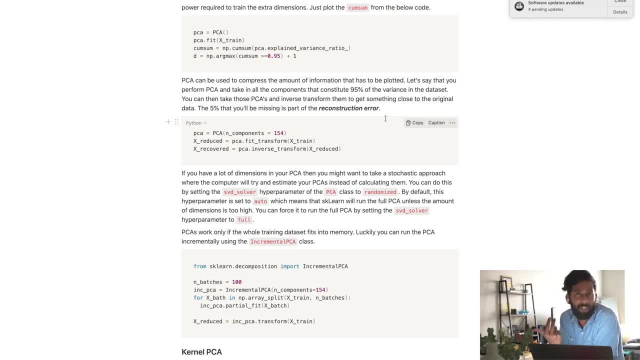 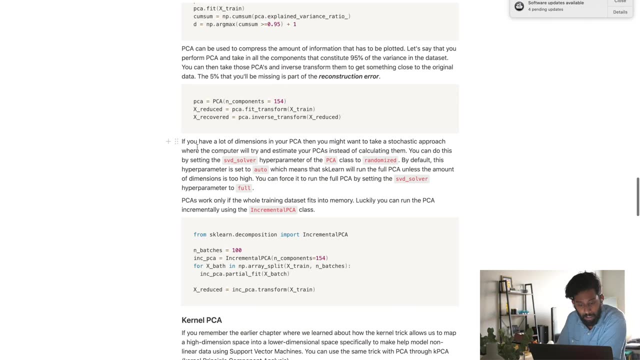 You can do an inverse transform and say, okay, I want a 5% reconstruction error, I want a 3% reconstruction error. Basically minimize the reconstruction error that you want. That's another method that you could use. So if you have a lot of dimensions in your PCA, 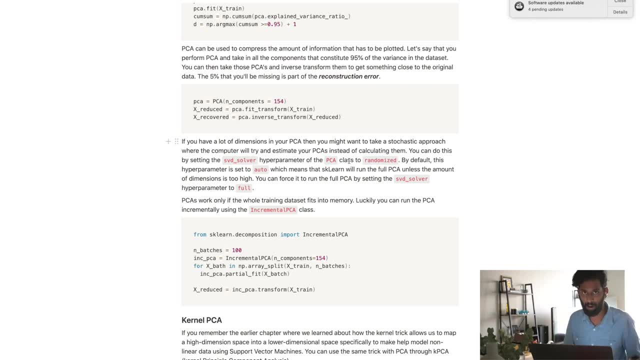 then you might want to take. If you have a lot of dimensions in your PCA, then you might want to take a stochastic approach, basically non-deterministic, where your computer will try and estimate your PCAs instead of actually calculating them. And you can do this by setting the SVD solver hyper-parameter of the PCA class to randomize. 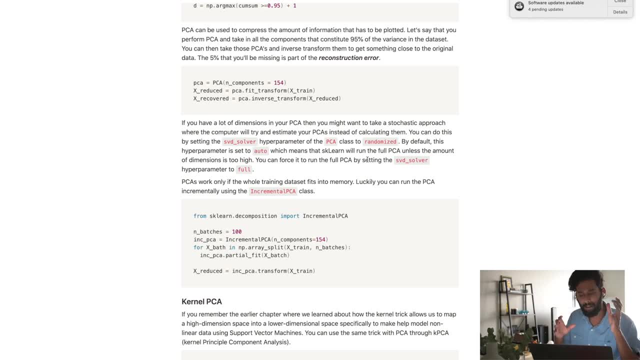 And by default, this hyper-parameter is set to auto, which means that the logic is a little bit complicated, But basically it takes a look at your data and it uses a rules-based method to determine whether it should use a stochastic approach or a deterministic approach. 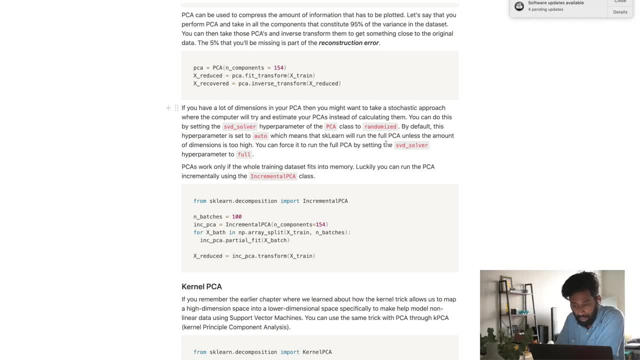 So it's normally set to auto And you can do this by setting the SVD solver hyper-parameter of the PCA class to randomize, And what happens is SKLearn will run the full PCA unless the amount of dimensions is too high. if you have auto on, and then you can force it to run the full PCA using SVD solver with the hyperparameter set to full. 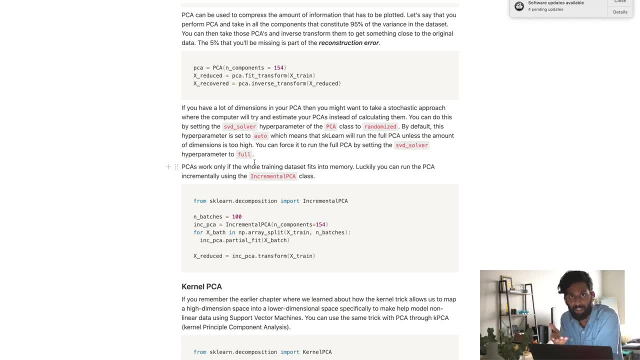 And the reason this is important and it's not something I can really demonstrate with the amount of data we have today, because there's too little data. It really needs to be a massive amount of data. The reason you might want to do this is that a PCA can take a long time to solve if you have enough data or if you have a weak enough machine. 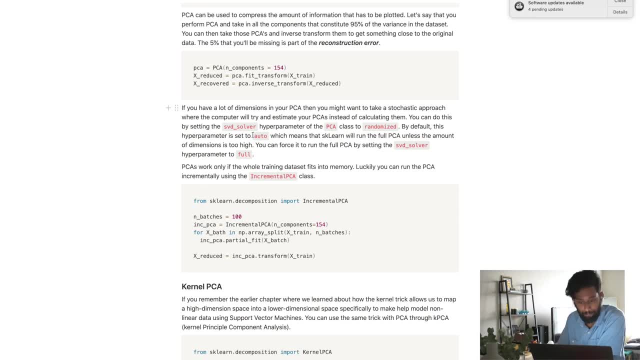 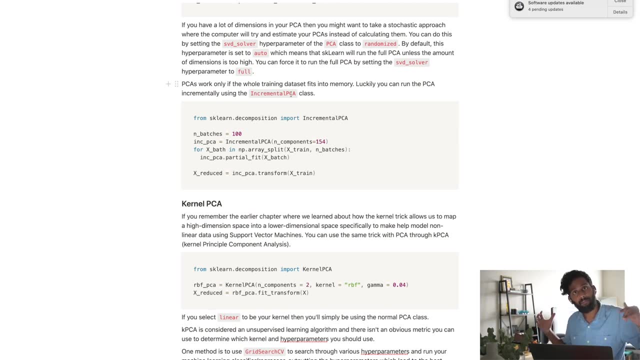 So this is why you might want to use the SVD solver method, or hyperparameter, I should say. And then PCAs only work if the whole data fits inside the memory of your computer. Again, this isn't enough data to actually demonstrate that with, but you can use the incremental PCA class in order to actually reduce the amount or in order to, sorry, incrementally feed that data into your computer. that way you can fit it into memory. 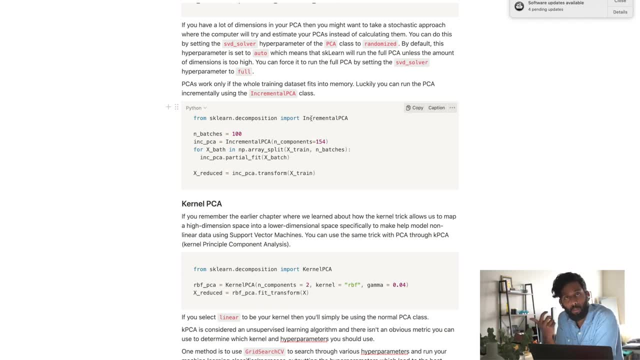 And you'll see this is one of the problems that data scientists really start encountering. at one point in time, too, The amount of data they start working with is so massive that just the limits of the computational power they have really start to hit. I personally have not worked with that much data in a machine learning context. 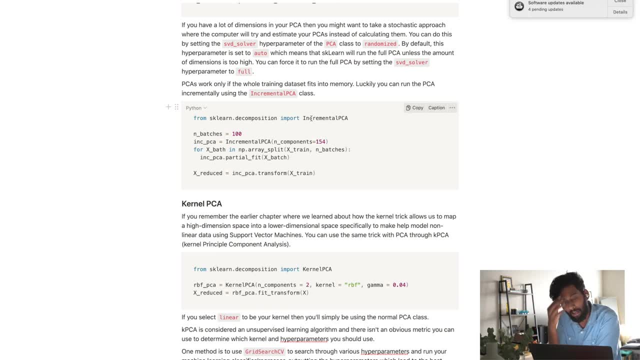 And there was one Kaggle data set I wanted to use. There's this really cool four gigabyte data set that Jane Street- for anyone that doesn't know where Jane Street is- is a hedge fund. I guess It's some major New York Wall Street firm that they do all kinds of computational training. 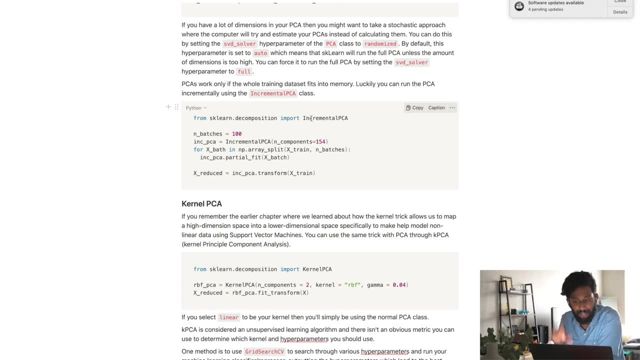 It's stuff they use. that's really really cool. And they have a competition on Kaggle where basically they released a four gigabyte data set with 100 features or something And they say, okay, Predict the stock market with this. It's really interesting. 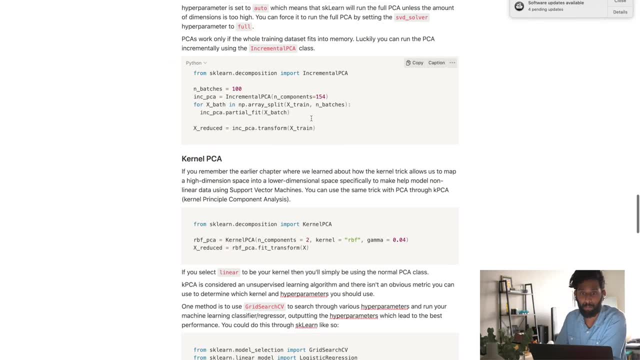 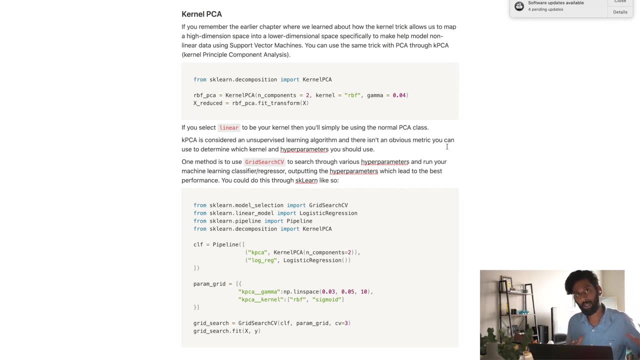 The prize money for winning that is $100,000.. So if you're interested, go check it out. But the submissions are over for now. So if you guys remember in the earlier chapter where we were talking about the kernel trick- I think it was when we were talking about support vector machines- 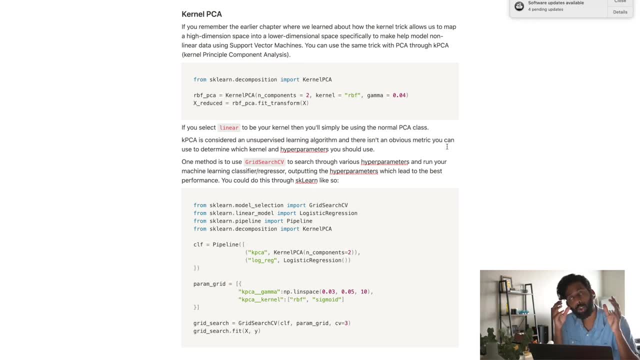 If you remember, the kernel trick was just a method by which we could transform a nonlinear set of data into a format that a linear algorithm, such as support vector machines, could actually handle, And that's why we We can apply that exact same logic to something like PCA. 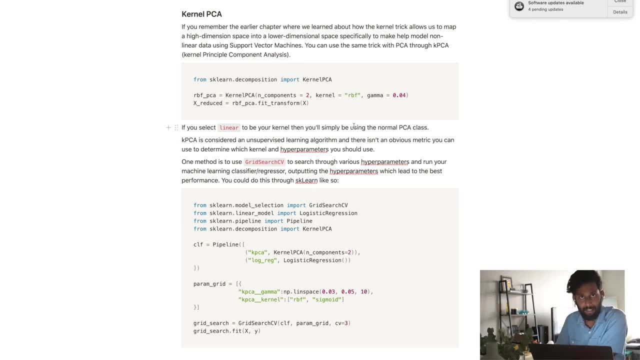 And it's called kernel PCA. So what happens is what we've been running so far is basically a linear PCA, But we can also run a kernel PCA on RBF or using a sigmoid kernel. There might be more kernels than that, but these are just the ones that we have back. 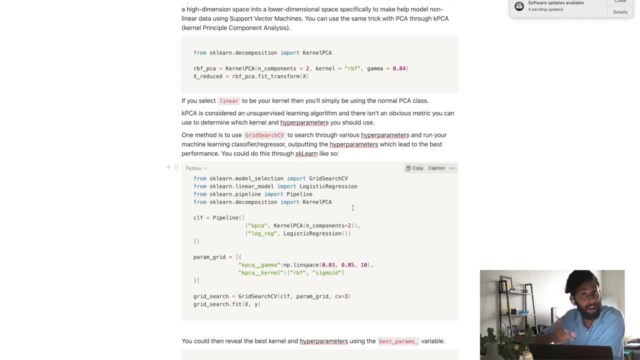 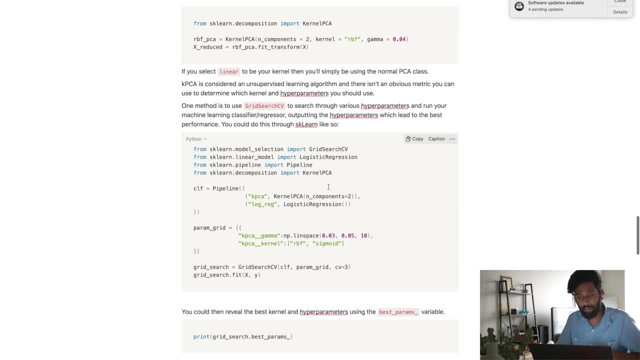 These are just the ones that I read about inside the book. So what happens is: if you, We can, If you. There is. One problem that they note in the book is that there's not necessarily a set of rules that tell you: okay, like you want to run this kernel with this gamma on your data. 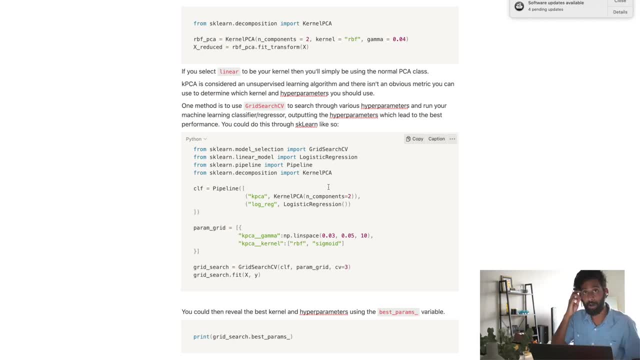 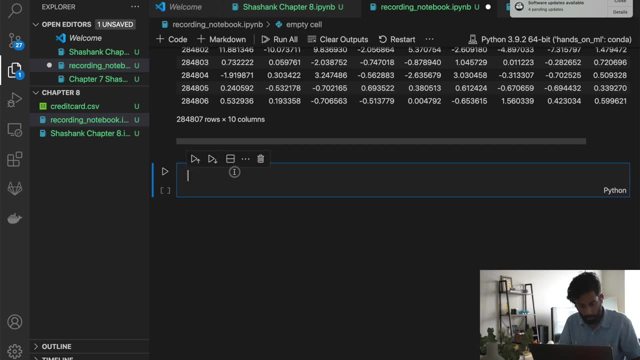 And because of that, you might just want to use grid search in order to actually determine, okay, which one has the best parameters. And if I copy this code over here, then you'll see. I'll put it over here And let's run it. 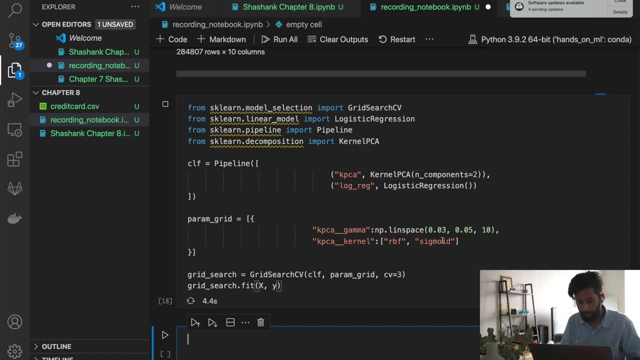 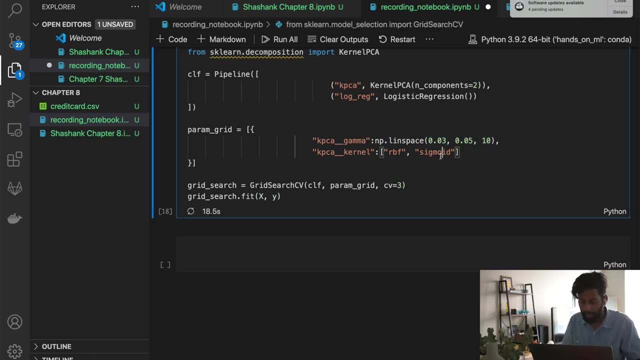 It'll do a grid search on. It'll do a grid search on using both the RBF and the sigmoid kernels And these, And then, basically, for anyone that doesn't know, nplinspace is basically a NumPy method that creates a range of values based on, like how you decide to write the method. 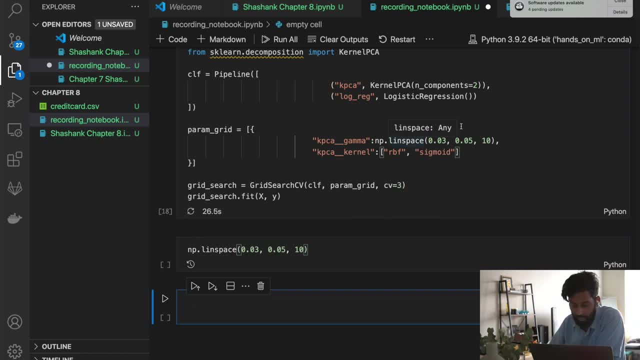 So, like I'll run this right afterwards, I'll show you how this one works. So it's testing out all these gammas and it's testing out all these kernels, And what it's doing is it's running a kernel: PCA. 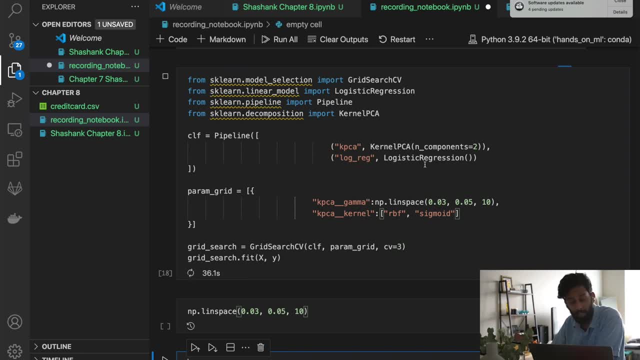 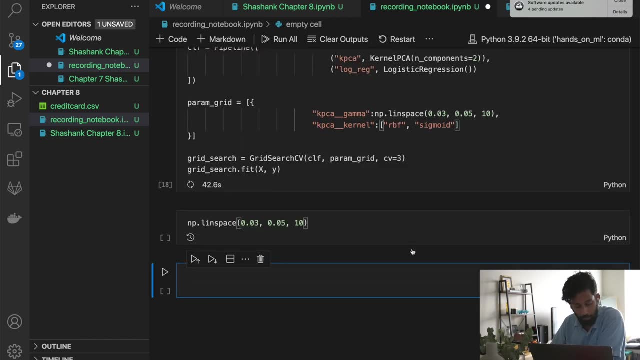 And then a logistic regression to try and classify our data And then telling us, okay, like which one gives us the best? Which one has the best parameters inside it? So, as you can see, this is actually taking a little while to run, because the amount of data I have is actually quite large for the purposes of what we're running right now. 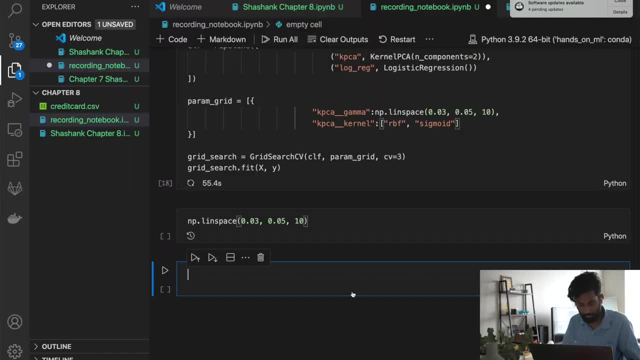 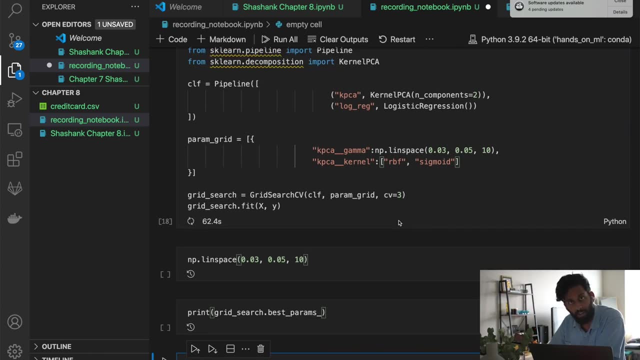 And we'll leave that to run while I copy this over here. And basically this is kind of just like brute forcing, trying to figure out, okay, like what are the best? What are the best, What are the best parameters for us to run? 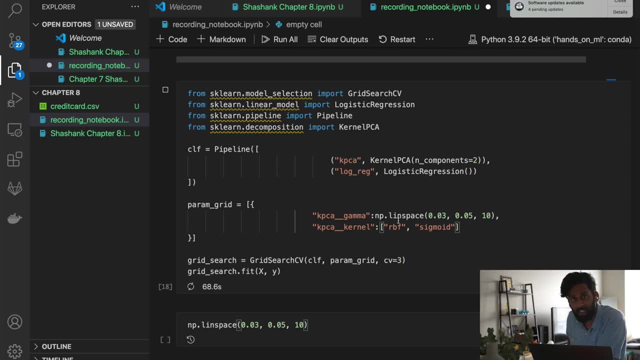 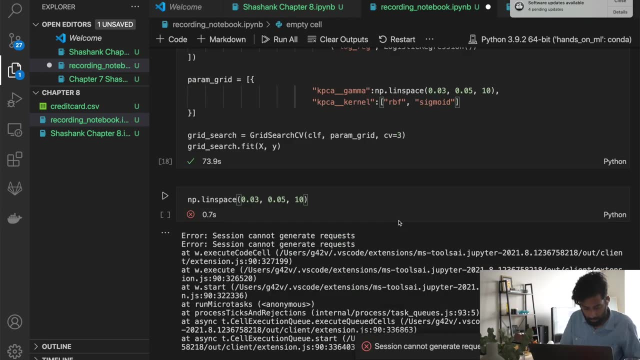 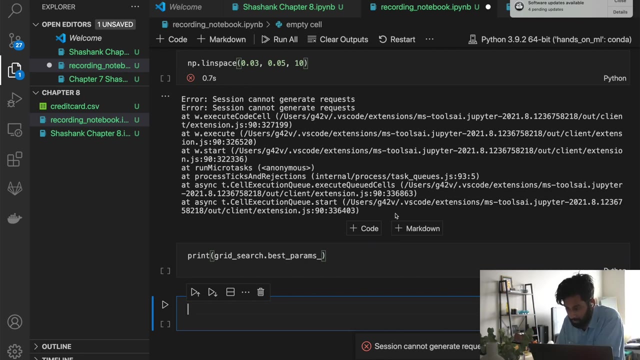 And remember a logistic regression. although it's called a regression, remember, it's actually a classification algorithm, Very confusingly named, but it's a classification algorithm, not a regression- one Interesting. So this might just be a problem with too much data. 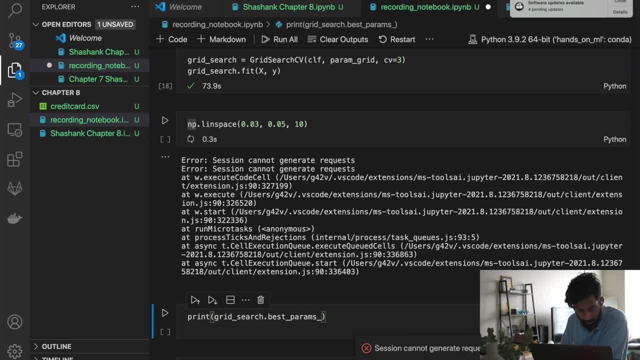 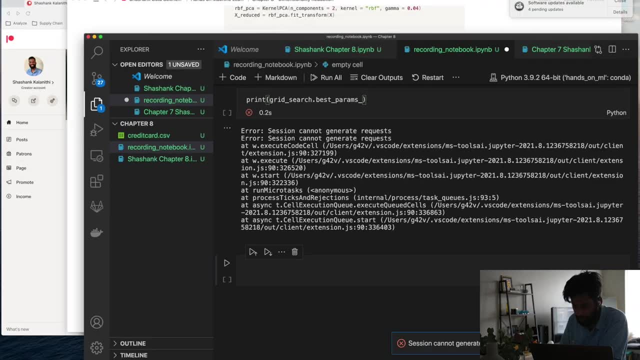 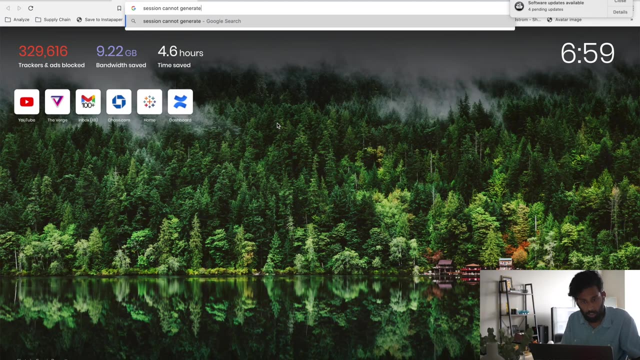 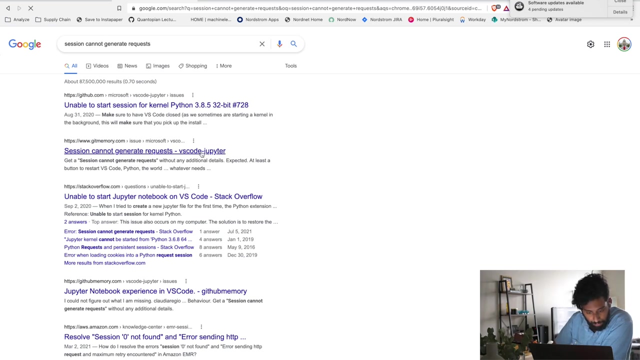 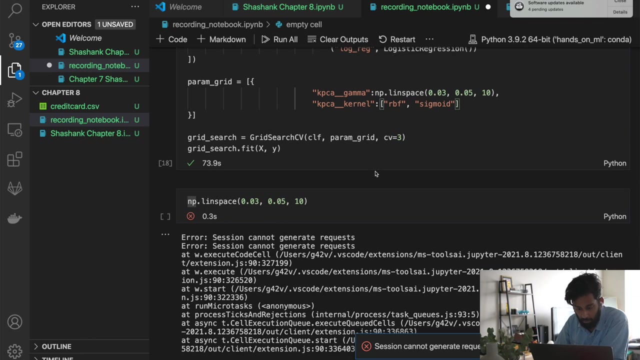 Cannot generate requests. Session cannot generate requests Interesting. Generate requests Interesting. It just looks like it's some error, So that might have been too much information for it to handle. Oh, I think the entire kernel crashed Like the Jupyter kernel. 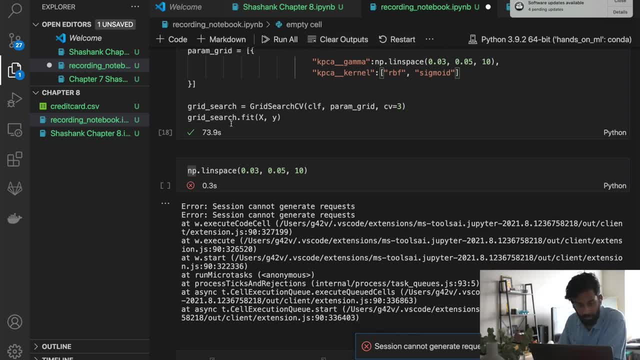 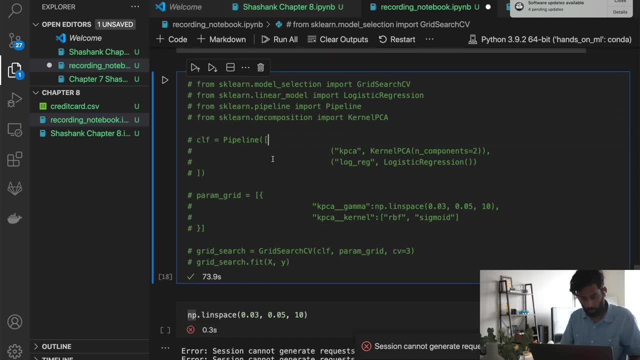 Yeah, not, Not like RBF or Sigma. I think my Jupyter kernel crashed, So I'm going to get rid of this, Or you know what. You know what we could probably do. Check this out, So let us. 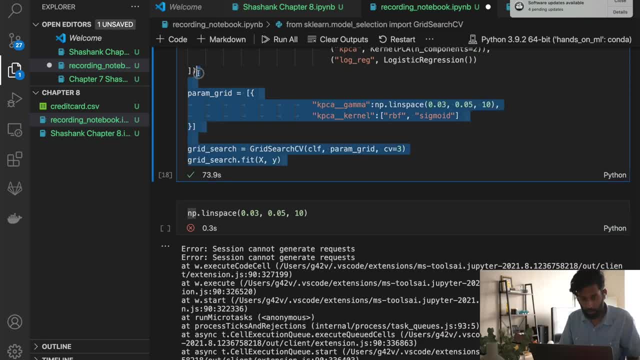 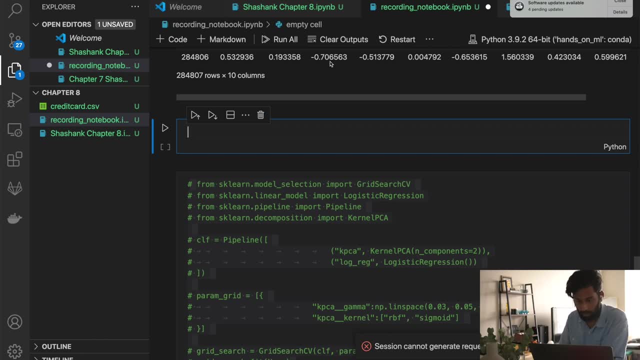 Let us comment this out That way. it doesn't run right now And then run everything. Session cannot generate: Yeah, so the entire thing crashed. Oh, it's gone. Okay, so I have to restart VS Code, So let us quit this. 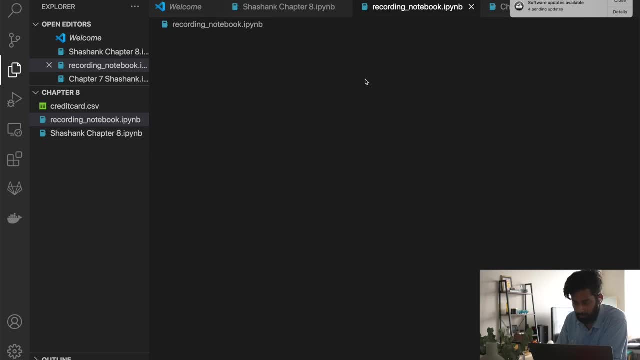 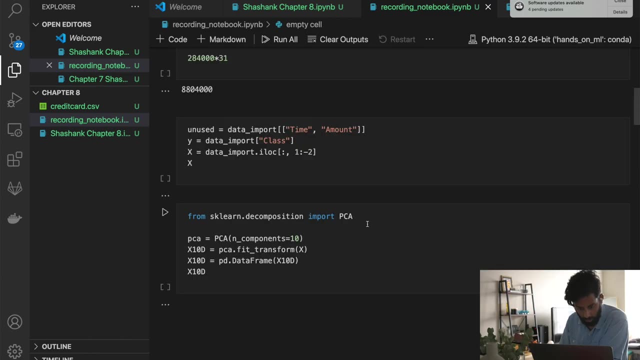 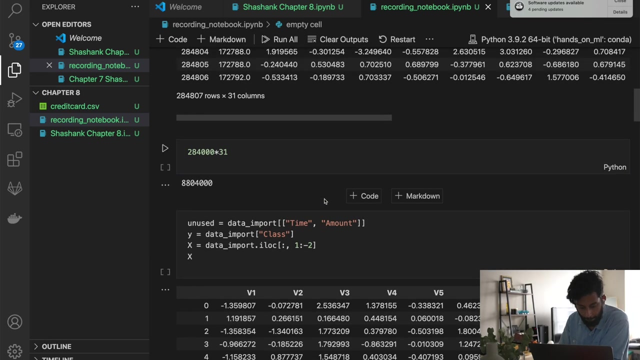 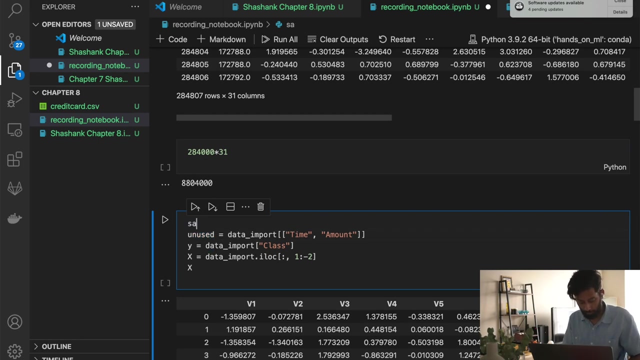 And then run it again. So what I'm going to do now is I'm just going to sample the data And hopefully that will Interesting. Hopefully that will make it to where we can actually run this without crashing the entire thing again. Data import- dot sample. 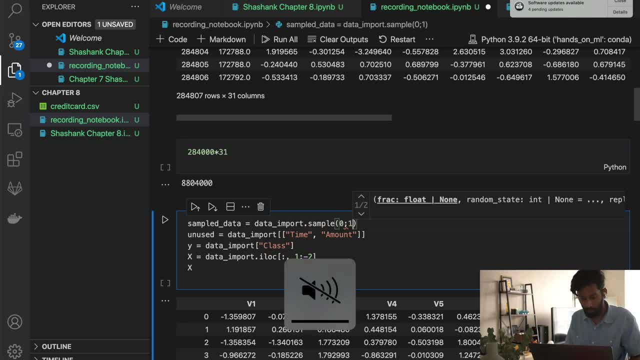 So, basically, it'll just take a random sample and let's just say we want to sample 10% of the data- 28,000 should be more than enough- And then let's go ahead and replace that, replace that, replace that. 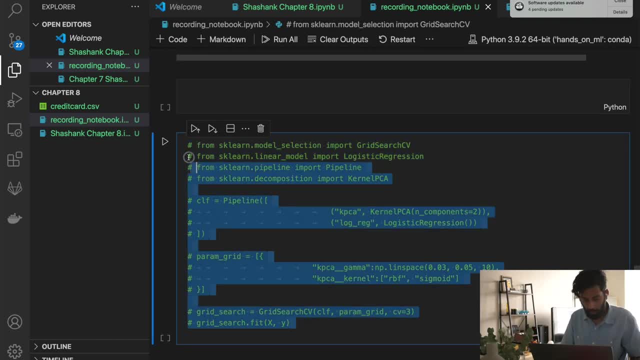 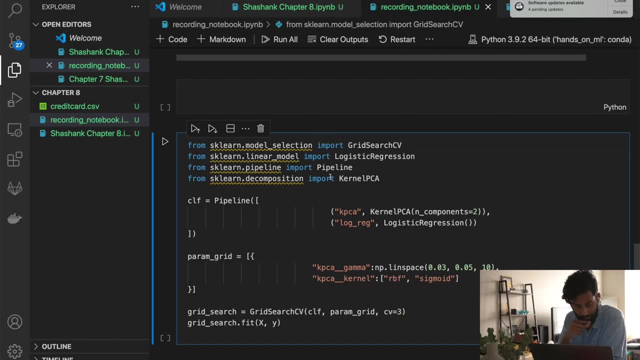 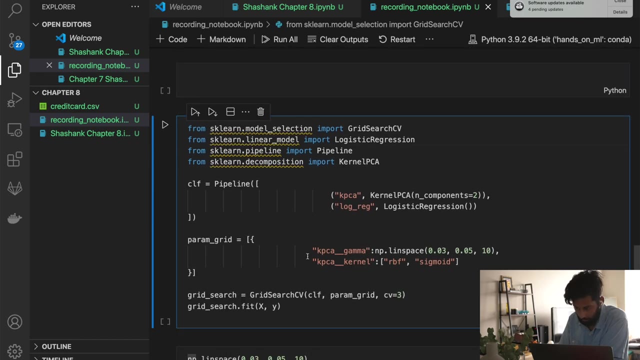 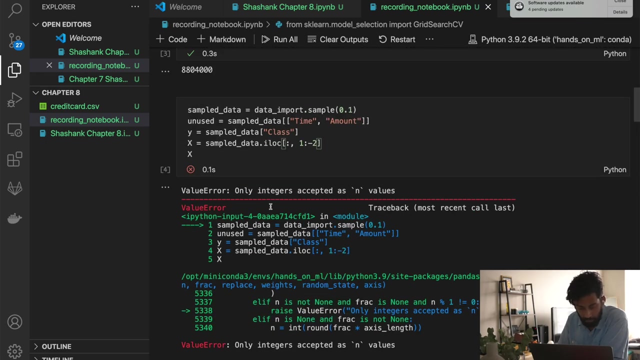 And then we will uncomment this Save and then run everything. Okay, so now we're going to go ahead and run this, and then we're going to go ahead and run this. Oh, it crashed over here. Only integers selected as n value. 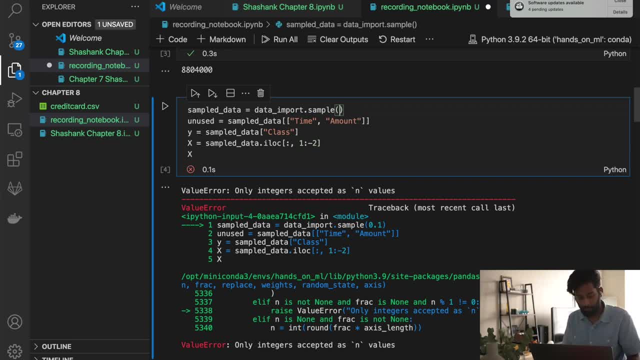 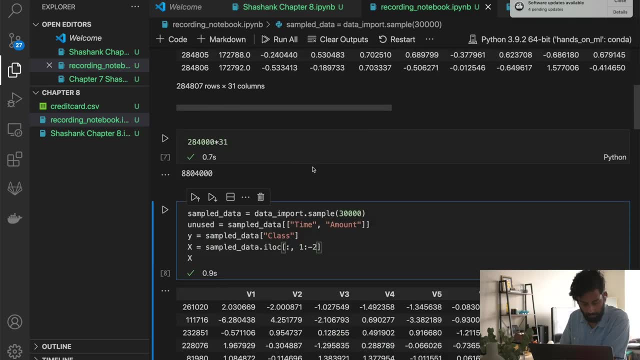 I thought I could put a float in here. Okay, so let's just do 30,000 records and then we'll try it again. There we go. Okay, we've sampled our data- 30,000 rows- And let's see if we have a crash over here again. 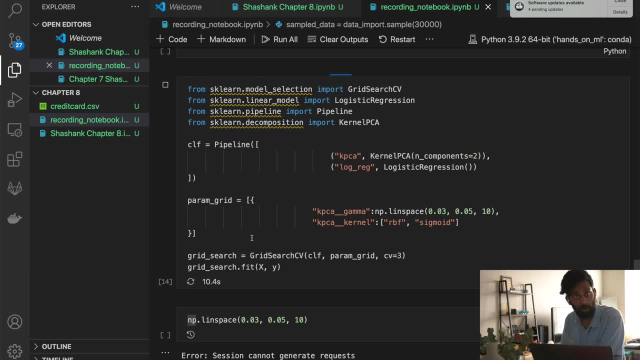 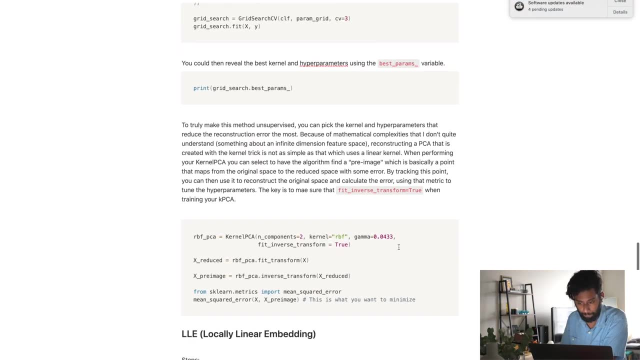 So it is running again. It's running with about 10% of this, It's running with about 10% of the data, so hopefully this leads to better outcomes than before And let's see what we have next before. Oh, I guess we can go over this while that's still running. 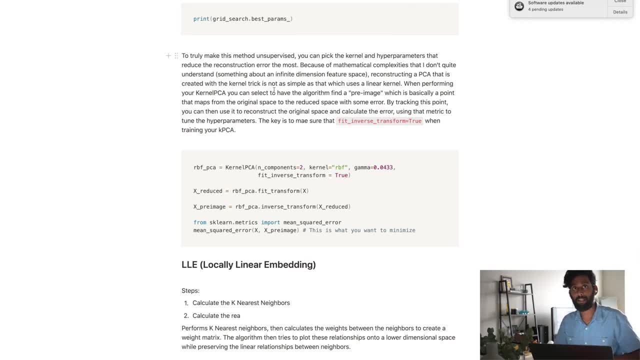 So, in order, if you want to make this method truly unsupervised, where basically it picks everything for you, you can pick the kernel hyperparameters that reduce the reconstruction error the most, And because of the mathematical- and there's some like in the book, there's some mathematical- 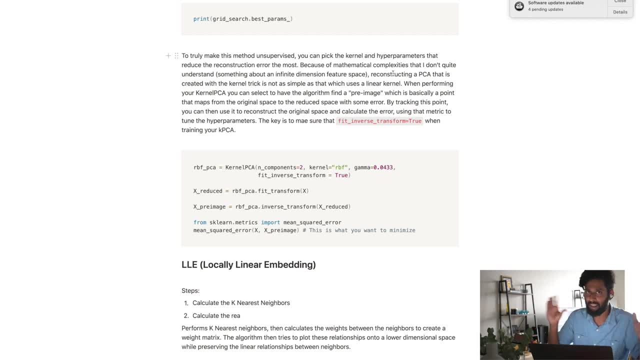 complexities that I don't quite understand, something about there being like an infinite dimension feature space. You can't- You can't perfectly reconstruct a kernel, PCA. I'm guessing it has something to do with the fact that, like, you can transform the data with a kernel, but you can't fully transform it back. 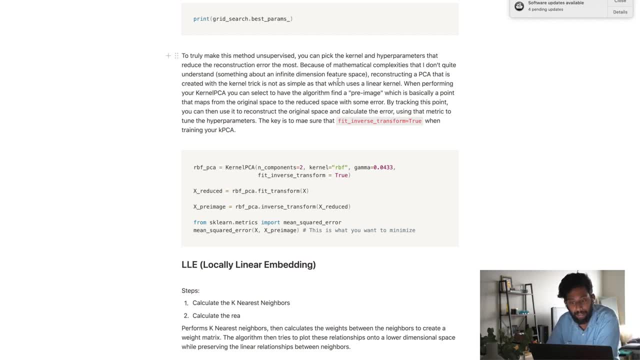 And you kind of have to like estimate the backward transformation, And what happens is you can. my understanding of what they're saying in the book is that whenever you want to inverse transform it, what it does is you have to specify the fit inverse transform method in your kernel PCA. to be true. 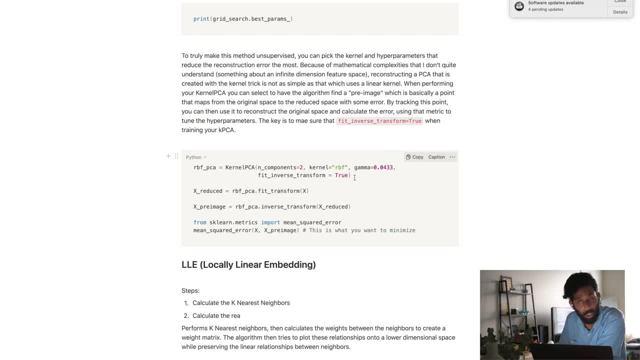 So you'll see your kernel PCA where you specify the inverse fit, Inverse transform method to be true, And once you do that it kind of track. it tracks one point from start to finish of this entire method And then it sees what is the deviation of that point from where it originally was. and 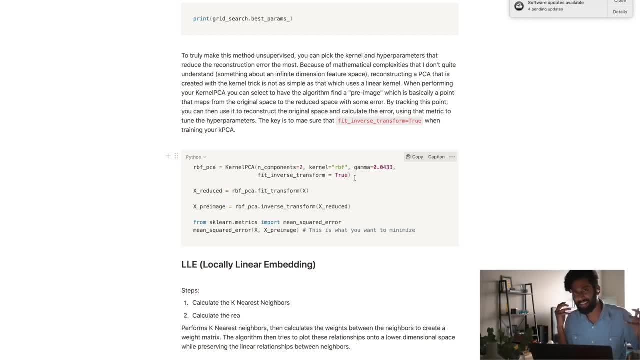 then uses that to estimate where everything else should go back to Again. the math and logic behind this part was a little bit complicated for me, But my basic understanding is that if you want to inverse transform your kernel PCA, then you need to make sure that this method it basically needs to track the point from- 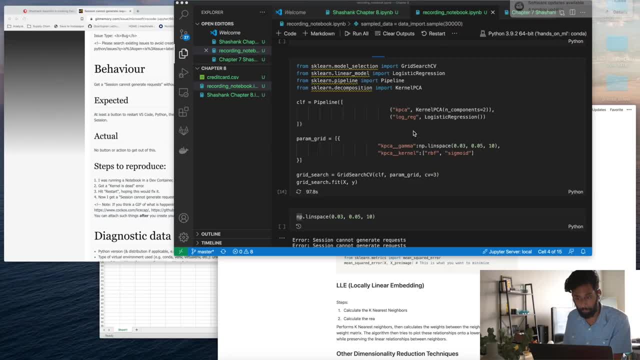 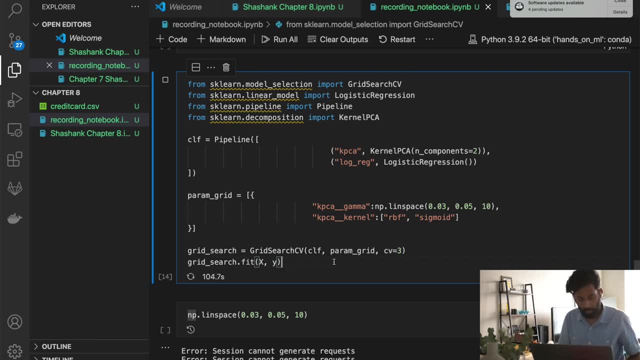 the beginning, which is why you might want this method to be true when you do it. Okay. So the fact that this is still running is not giving me a lot of confidence, But if it doesn't work, then we'll just skip over it and go on to the next section. 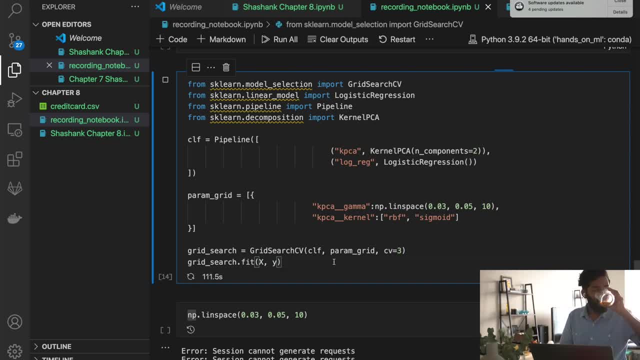 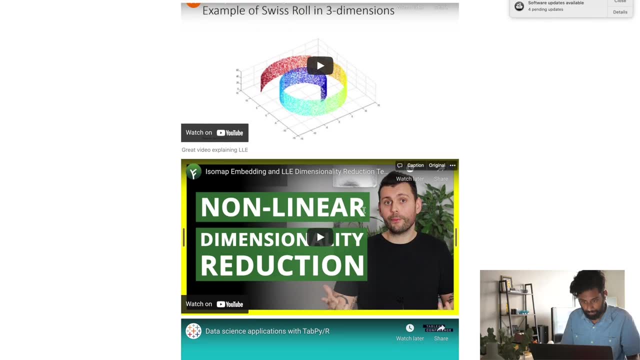 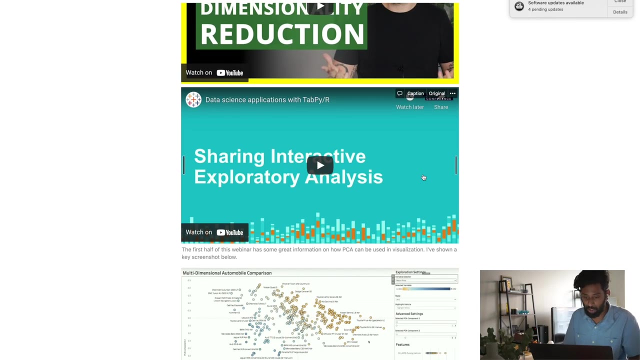 I have something a lot cooler I want to show you guys, anyways. And then, as usual, I have a couple of other sources inside my notes that are on my Patreon, where I just go over some of the other stuff, But some other sources that I think are also helpful in addition to this book. 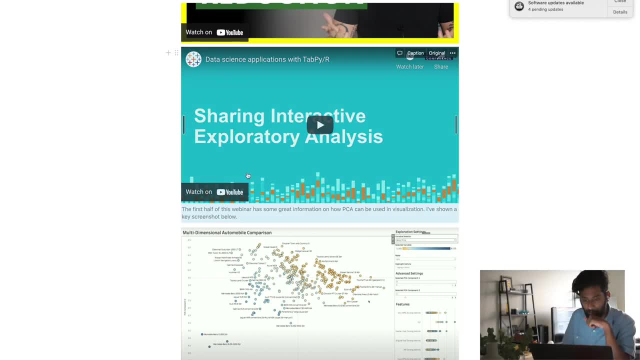 One thing I really want to show you guys is, if you look, make sure you look up this video by Tableau. So I went to a Tableau conference a couple of years ago and okay, so it looks like it's not loading. 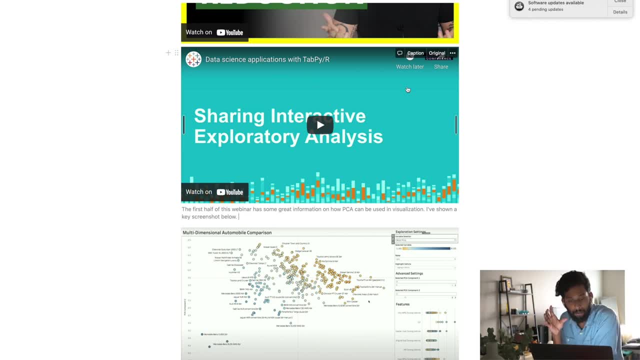 But I went to Tableau conference a couple of years ago and they had this talk called Data Science Applications with TabPi and R. So Tableau is a BI tool. basically it's a visualization tool, more or less, And TabPi is a way to connect Tableau to Python. that way you can execute machine learning algorithms. 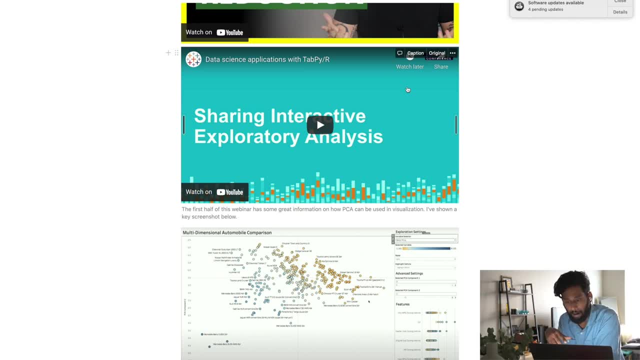 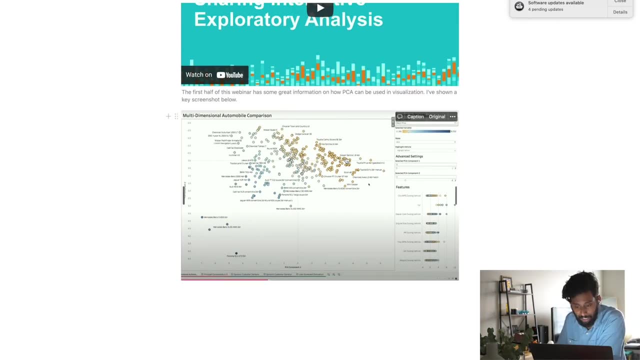 dynamically And display the results in Tableau. And they had this really cool demonstration over here on a PCA- I highly recommend watching this video- And they took this car data set right with like 10 different dimensions of like engine size, reliability, quality, stuff like that. 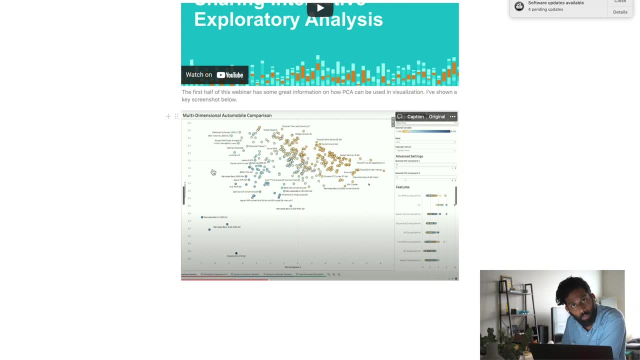 And what they did is that they demonstrated that PCA is a tremendous way to actually plot data that are maybe on 10 different dimensions onto a two-dimension plane, And what you could do with it is that- and this might be a little bit hard to see- let's 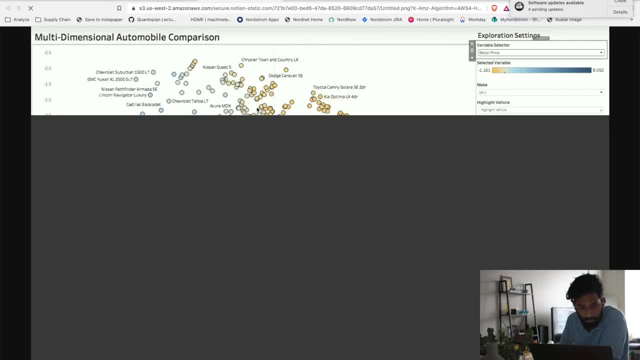 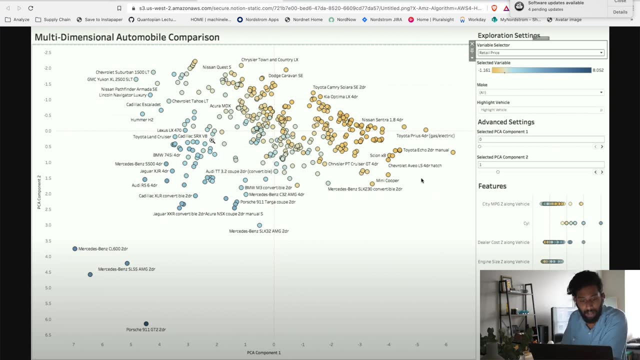 see if I can show you guys the original. What you guys can see over here is that they actually were able to reduce those 10 dimensions into just two dimensions and then label every single point. And when they did that, you could start to see patterns with where, how you could like. 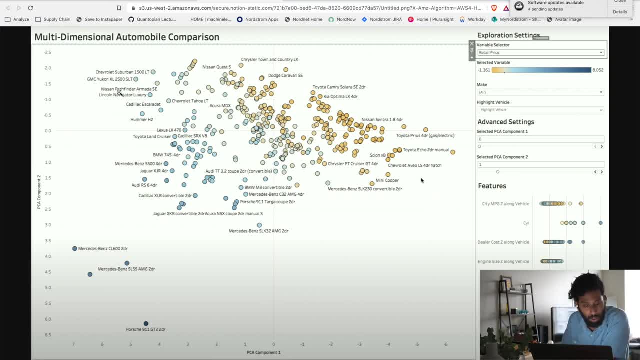 group your data. So, for example, you'll see Chevrolet, Suburban, GMC, Yukon, Nissan, Pathfinder, Armada, Lincoln, Navigator, Luxury. These are all massive American cars, or massive cars made for the American market, And they're all in this corner over here. 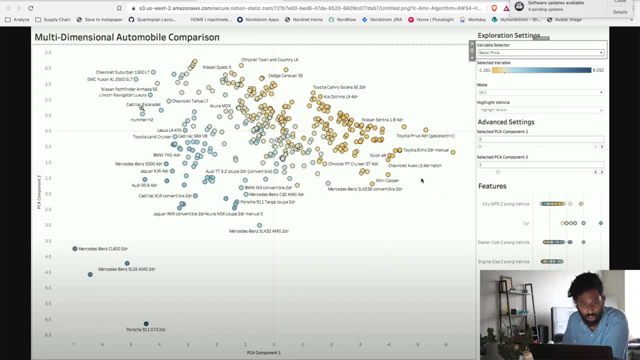 The Acura MDX, I believe, is an SUV. It's not a massive one, but it is an SUV. And even the Nissan Pathfinder. that's not an American car, but it is a massive SUV. if you've seen it And if you see the way the Nissan Pathfinder looks, you're like: oh, this was designed. 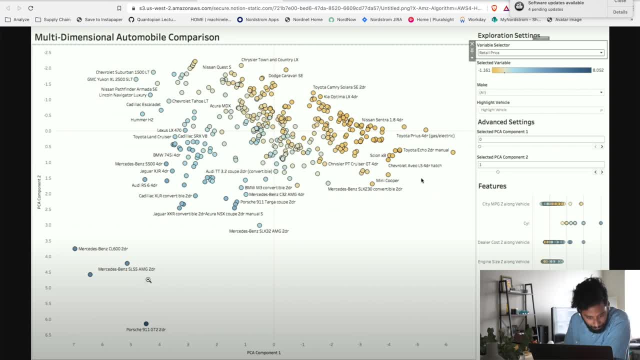 to look massive And you'll see, those are all in this corner over here, Really fast. German luxury cars are down here. So your Mercedes CL 600s, your AMGs, your Porsche 911s are down in this corner And I believe, yeah, you're really efficient. Asian cars: 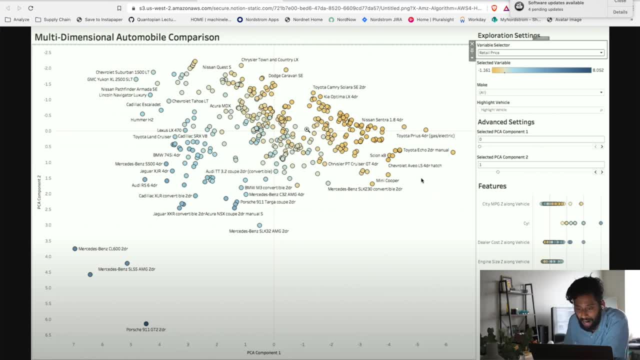 So Camrys, Kias, Nissans, Priuses are kind of in this area over here And this is tremendous Because imagine you're talking to a business owner or like someone in business that you need to talk to, And this is what really got me into PCA when I first saw it. 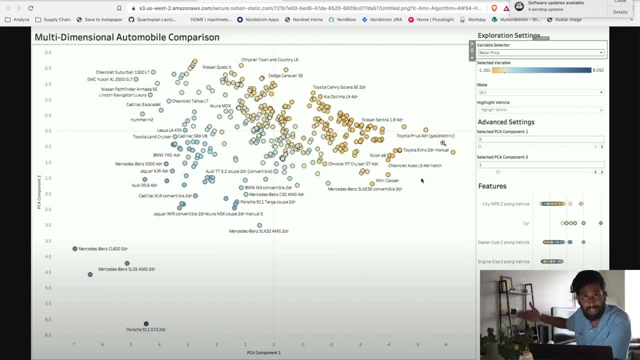 What they did is that they took 10 different dimensions or 10 different columns of data, crushed it down to just two. And this is something you can show to a business person and say like: oh, these cars are kind of similar. These cars are kind of similar. 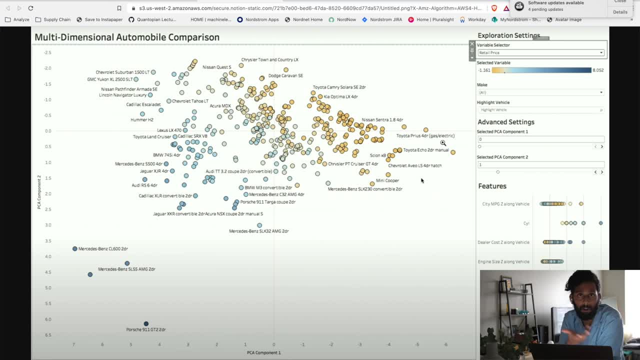 Now you're probably telling, you're probably looking at this, being like: oh yes, of course, massive cars are similar. These cars are similar to each other. Efficient cars are similar to each other. But what if this was something to do with customers, where the data was less it was? 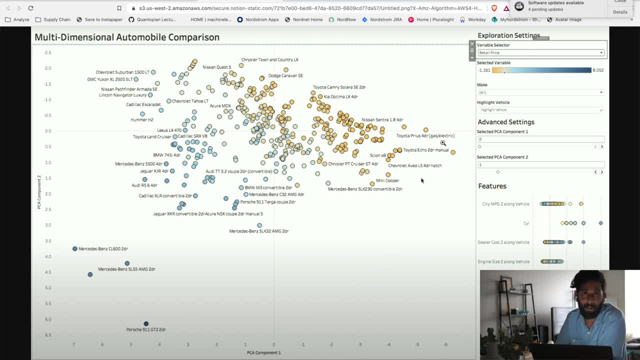 less obvious that that was the case. That's the beauty of PCA. That's one of the beauties of PCA. You can do two different things with it. You can reduce the amount of data you have to process for your machine learning algorithms. 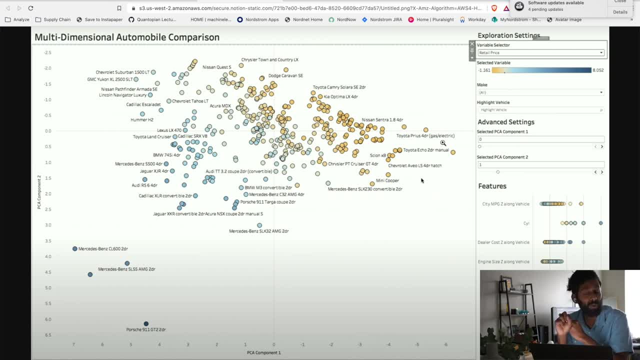 And you can reduce the data into two, three or four dimensions, which is something that can be plotted, And you might be wondering: how do you plot four dimensions? It's not you technically can, but what you can do is you can plot three dimensions and 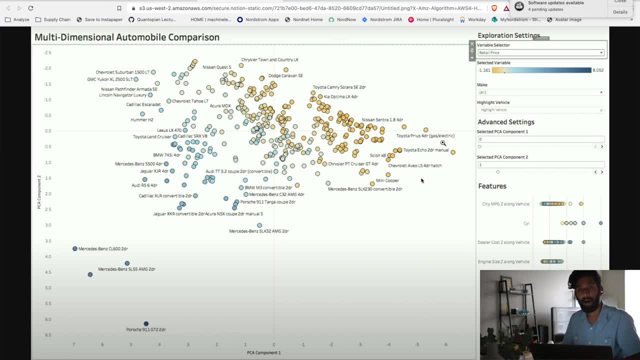 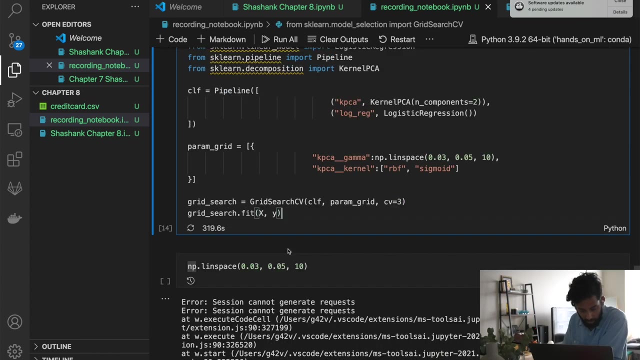 then color every single point And the color would be the fourth dimension. Okay, So for three years they did a two dimensional thing and then, you know, had the color be the value of the PCA. So, given that this is still running, I don't believe we're going to get some great results. 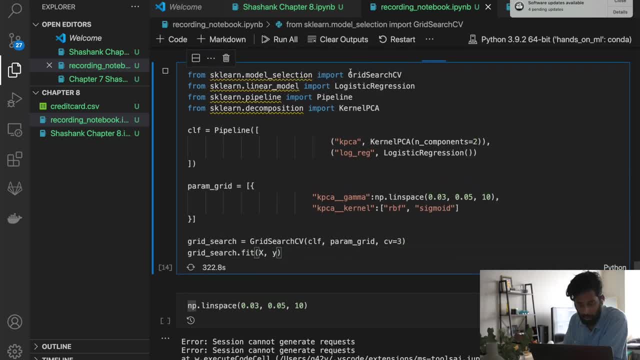 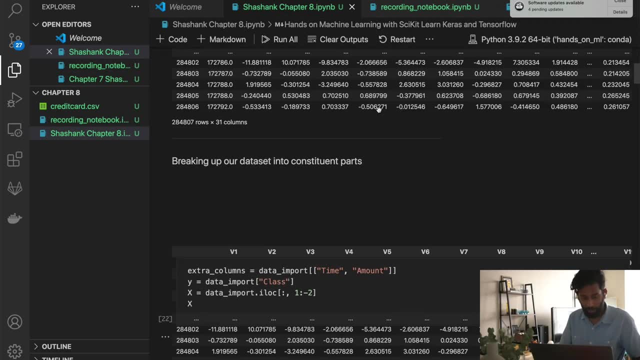 because we're at what? five minutes now, So I might want to just kill it, or we'll keep it running. And let me show you guys what I have in this notebook over here, And this is the notebook I have in my Patreon. but I'll go through the entire thing with 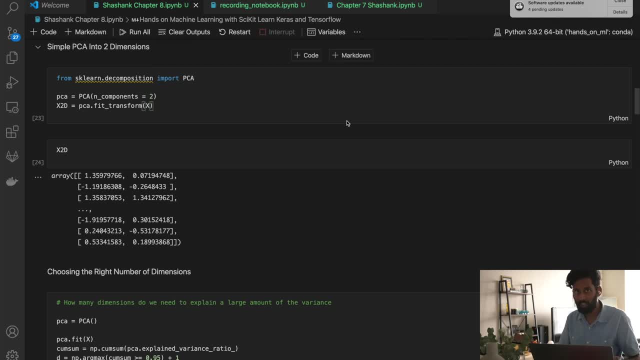 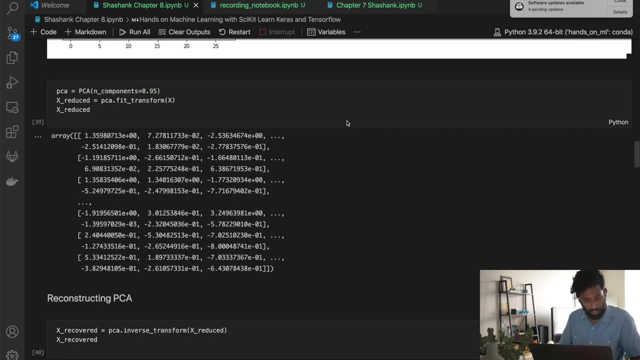 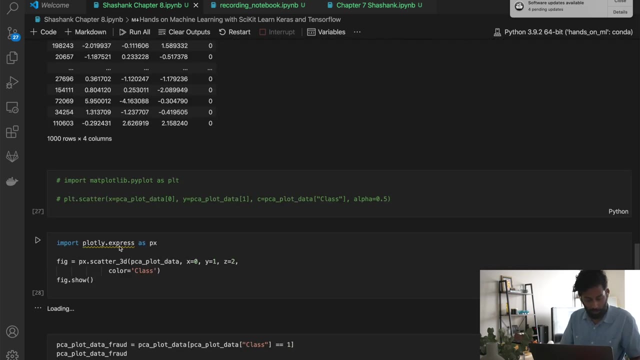 you guys right now. So it's the same basic stuff. The code's just a bit cleaner. I wasn't doing it live And what you'll see over here is as we go down. I have an entire section where I start plotting out the data and I start showing how you can use Plotly. 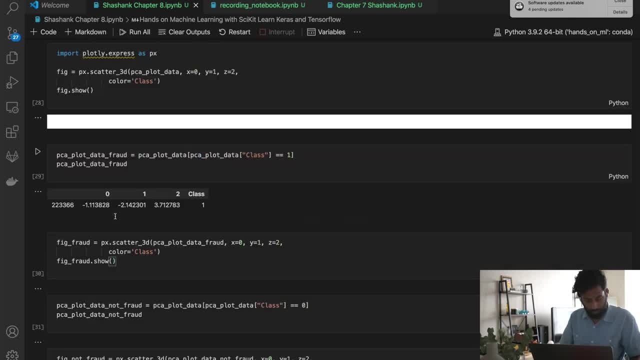 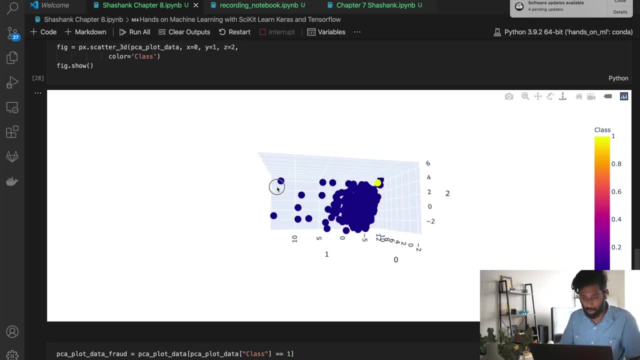 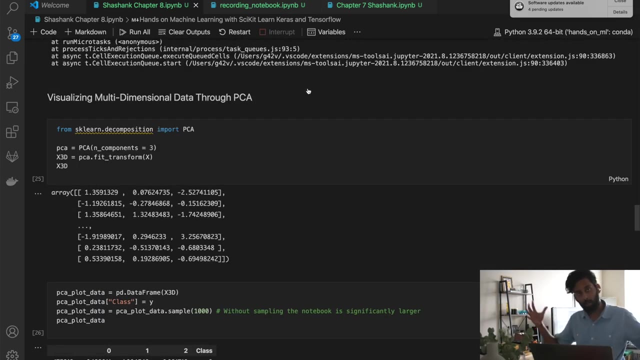 So to start plotting out data to show which transactions are fraudulent and which ones aren't. What happened is we took those 31 dimensions and then I crushed it down to just three, And then I colored the fraudulent transactions yellow and the non fraudulent ones blue. 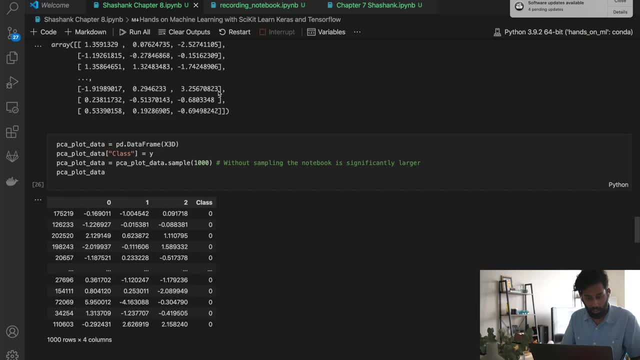 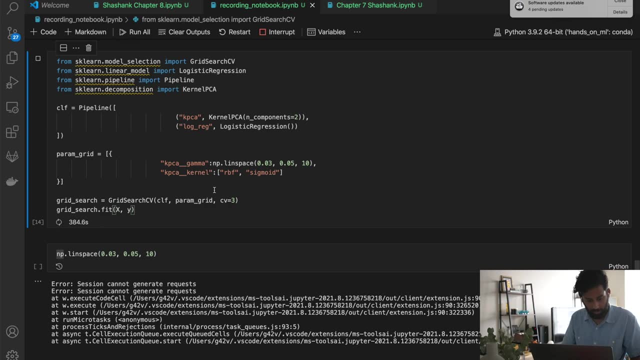 Oh, and this is just a sample, but let me go ahead and remove this sample method over here, So we'll do that. Save. This is still running. Let's kill it because it is. yeah, just hogging all the resources. 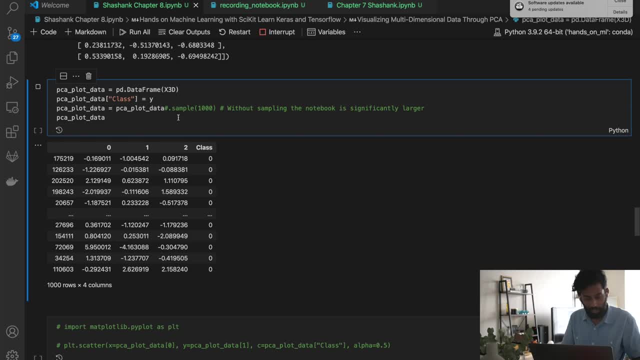 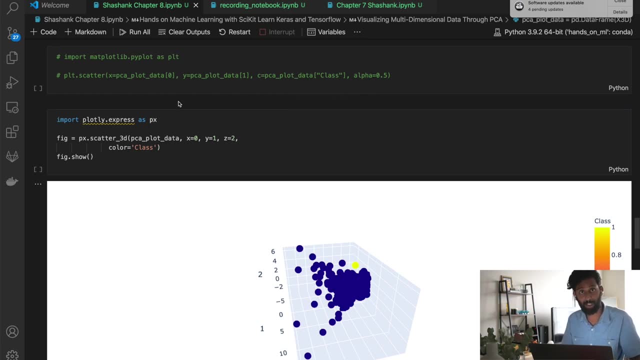 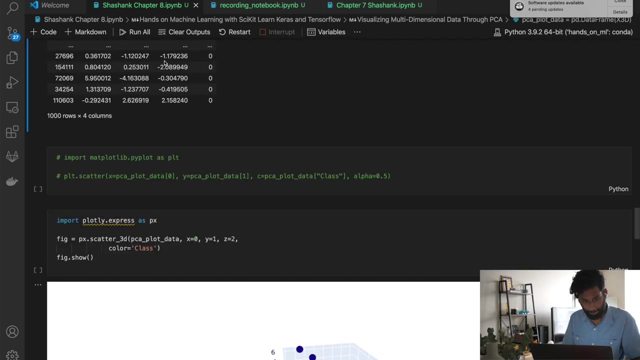 Run everything. Okay, Okay, Okay. And the reason I'm not live coding this is because you know I do want to. I think the video is stretching to about 45 minutes right now, What you will see over here If it decides to run. 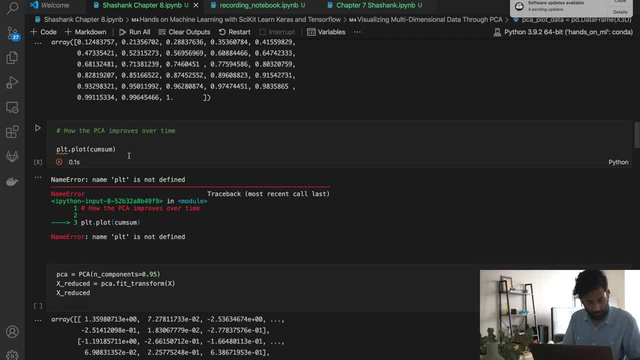 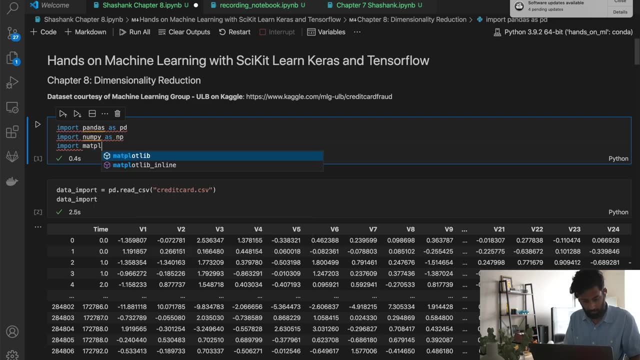 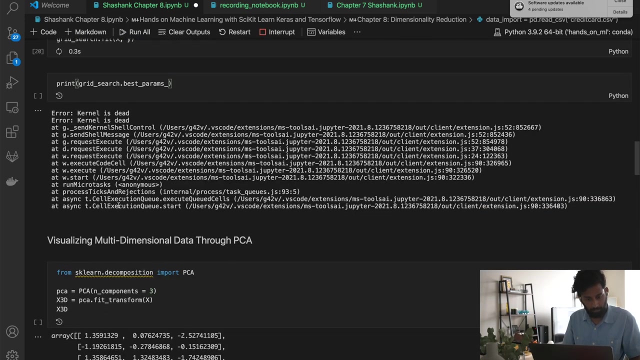 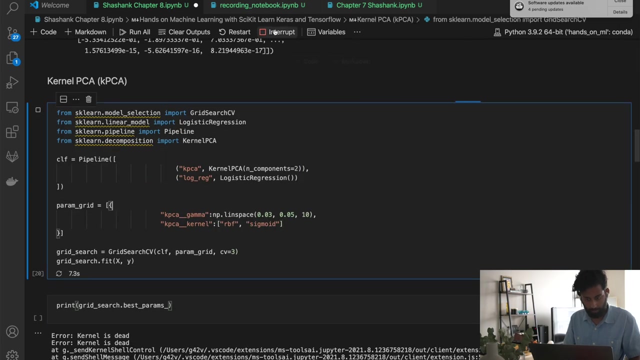 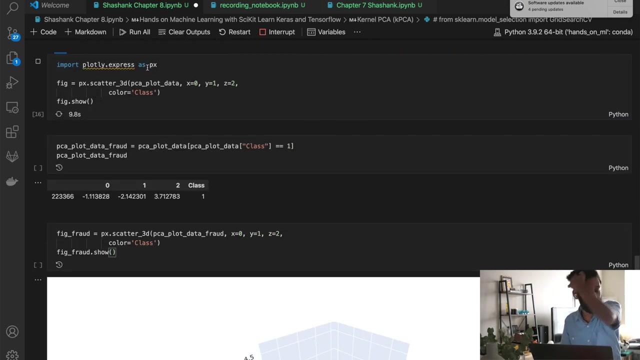 Oh, what error do we have? Ah, Okay, Okay, Okay, All right, Let's run everything now. Oh, shoot, Interrupted. I have the same code over here that I want to get rid of. Okay, So you can see over here. Plotly is now plotting the. 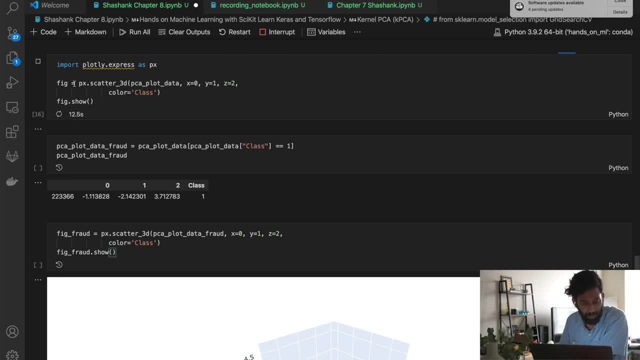 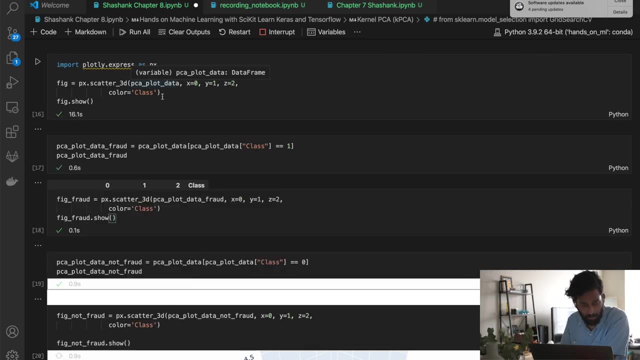 data And you can see. Plotly is super easy to use. You just import plotlyexpress as px And then you define your figure, which is pxscatter3d, And then you give your data set and then the names of your columns and then the color I want it to be class And 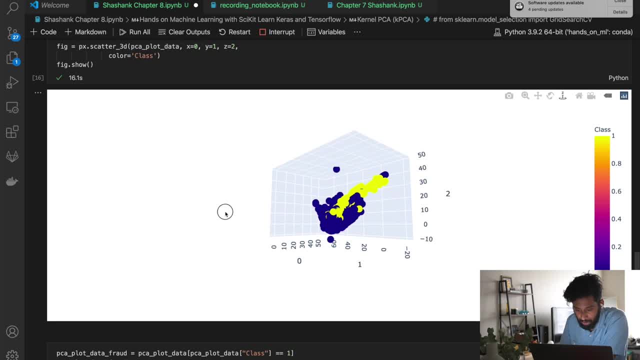 you'll see over here, yellow is fraudulent, Blue is non-fraudulent, And you can see it's very obvious that our fraudulent transactions follow a very specific pattern over here. I've taken 30 dimensions of data, crushed it down to just three And now I can show. 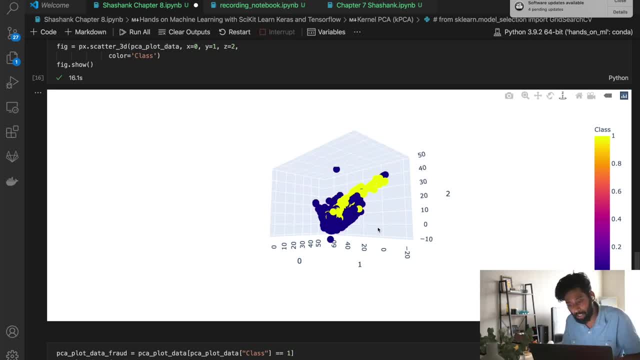 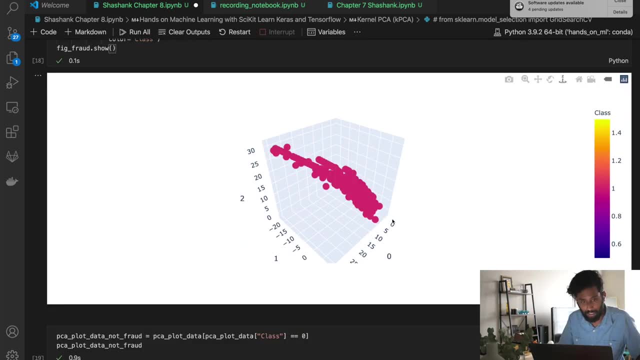 a stakeholder and I can say, hey, look at this, It's obvious. Our fraudulent transactions all fit a very specific pattern of data And if I wanted to plot this, is just plotting the fraudulent one. So you'll see if you look at this, this. 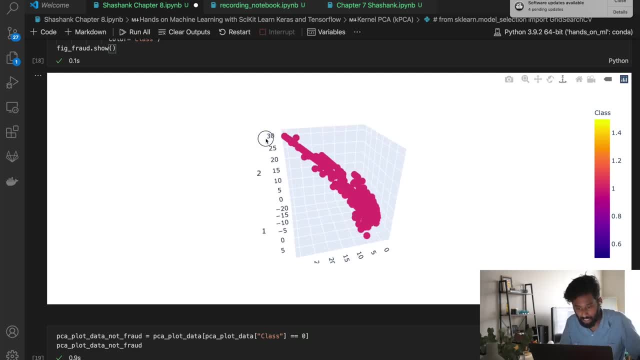 is just our fraudulent data. It's obvious that it follows a very specific pattern as to how fraudulent people decide to spend the money, or however fraudulent transactions work, And to me this is the big beauty of PCA And you can see non-fraudulent transactions. 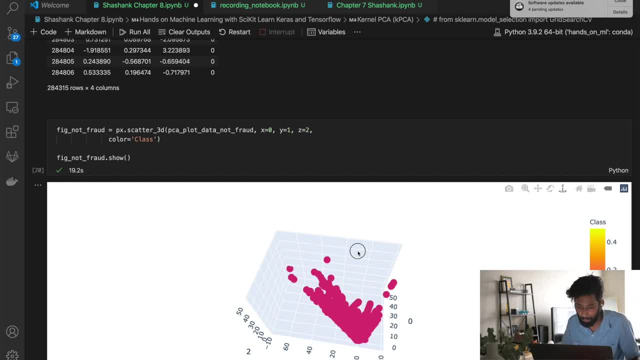 kind of have this V shape. It's a little bit hard to see because I didn't outline every single point. I would probably put this into a better visualization tool like Tableau or something, if I really wanted to visualize it. But this just gives you an example. 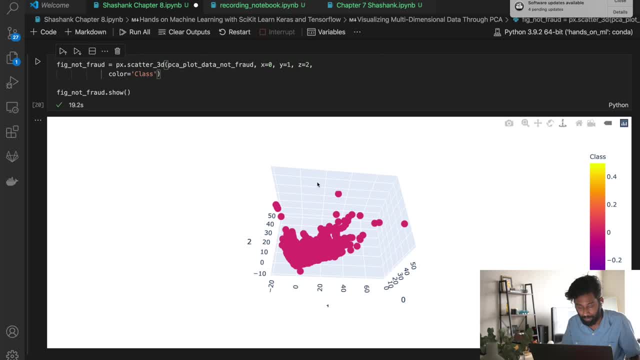 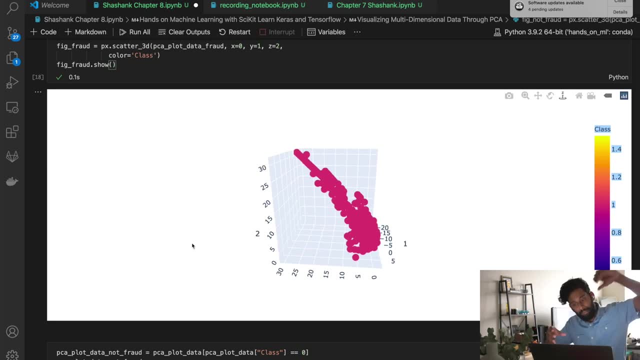 of how to handle that. But as you can see, probably more importantly than anything, it's obvious that fraudulent transactions follow this cone that starts down here and goes all the way up here, And then we can start breaking this down into smaller and smaller components. 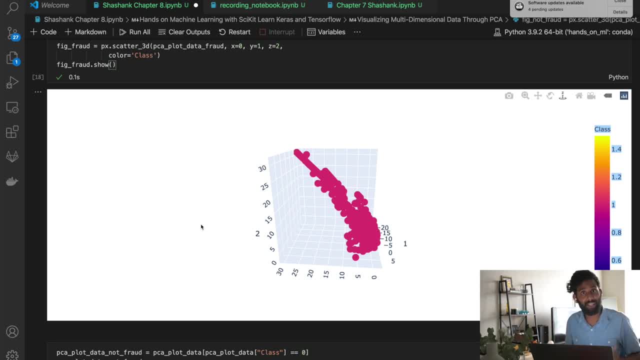 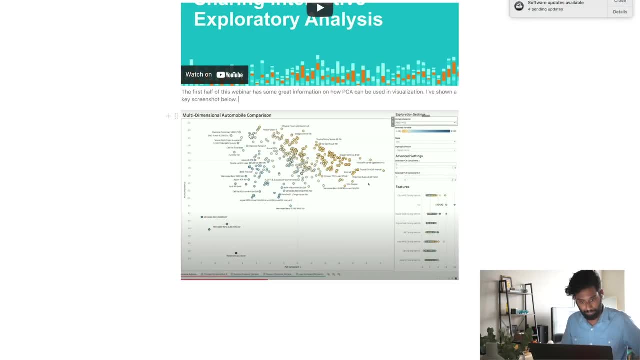 to explain which variables are the ones that are explaining that. So that's kind of what we're doing. That's, in my opinion, the beauty of dimension ality reduction and really what we're doing over here. And then finally they go over. 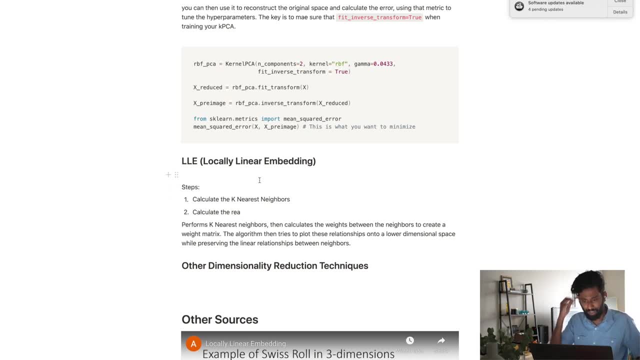 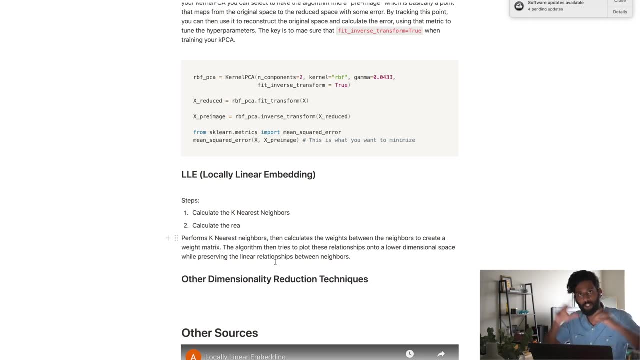 locally linear embedding. They don't really go over any of the actual concepts inside it. Basically, you just perform k-nearest neighbors and it tries to reconstruct the data through the relationship that every point has to every other point and plot all of that. 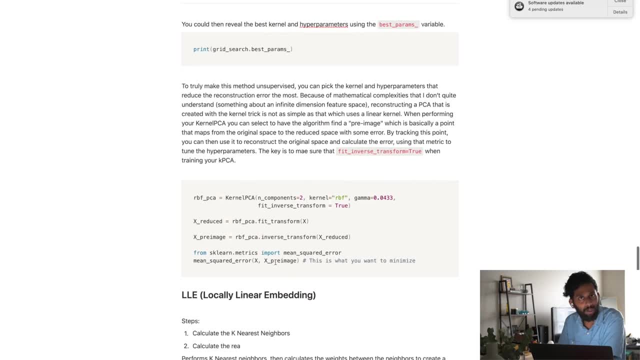 onto a lower dimensional space, But they didn't really spend much time on it. so I'm guessing that PCA is what they're doing, But they really want us to focus on. So that's chapter eight for you guys. I tried to bring. 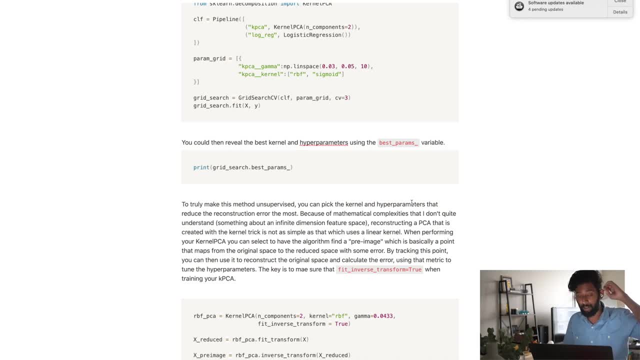 this video out a little bit faster And, as you can see, I'm shooting a little bit differently than I normally do. But if you have any questions or concerns, please leave them in the chat below. I'm trying to put out these videos a little bit faster than I normally do because 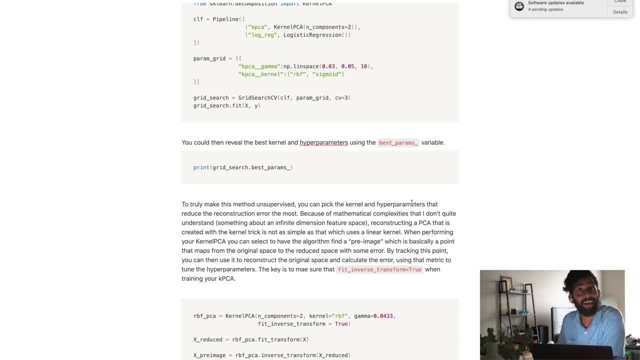 I really just love learning this stuff and love passing it on to you guys. But thank you guys so much for joining Again. if you haven't already, make sure to like, comment and subscribe in the video. It's a great way to support my work. Patreon is another great. 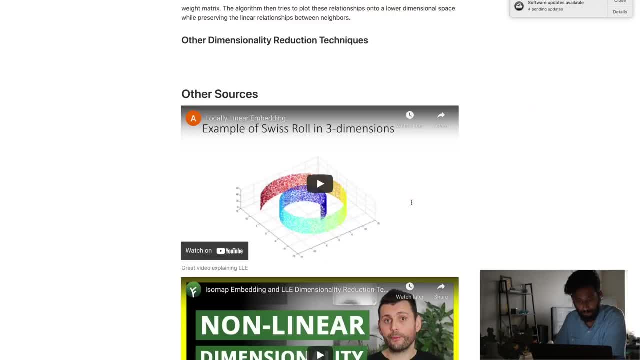 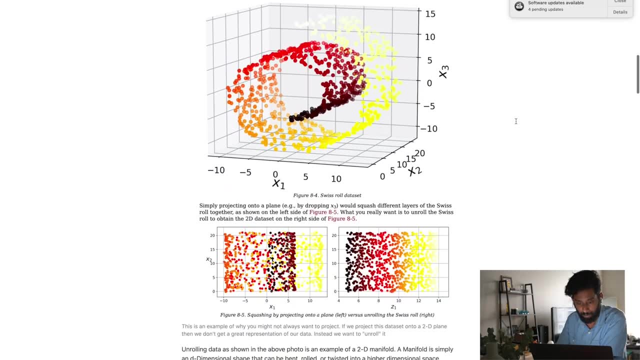 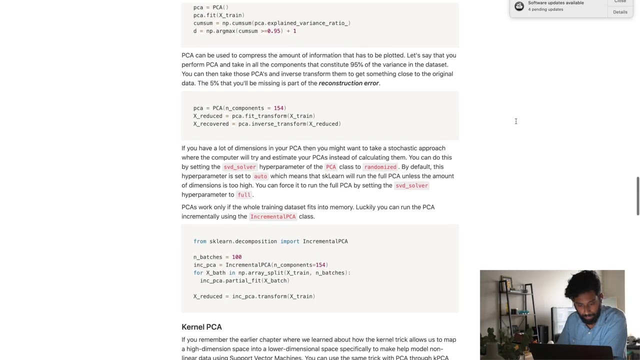 way to do that as well. The notes will be available over there, But, as you can see, I displayed all of the notes on this video. I'll just do a quick run through of them again, if you want to screenshot them for your own convenience, And then we'll do the same thing.